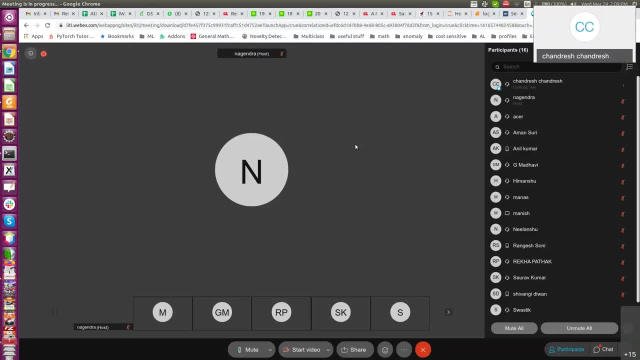 So if such kind of things are mentioned in the document, then you want to extract automatically, because manually it's not possible to go through all the literature, right? So what we will do is that you download the research paper, run this NLP tools and you want to understand. 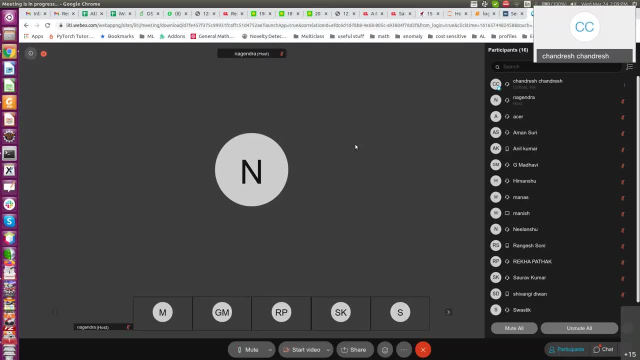 okay, What is the relation between the entities, between the coronal and the COVID, whether is there any effect relation or no effect relation, right? so that's an example of relation extraction and relation extraction. if you can do it automatically with minimal label, labeled data, then you are good. okay, so we'll see how can we build a classifier. 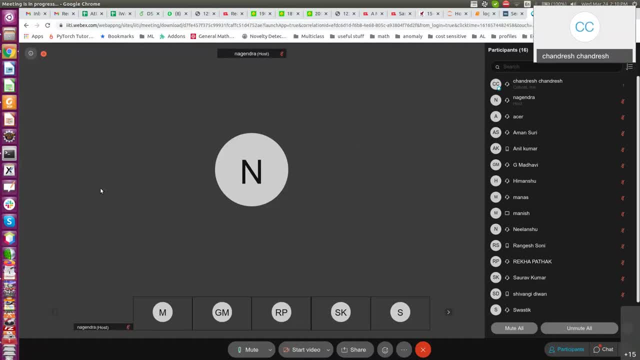 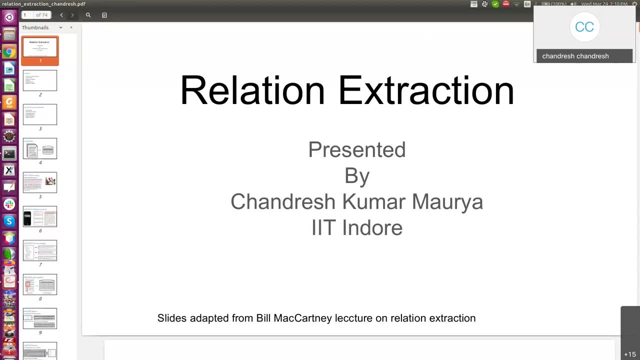 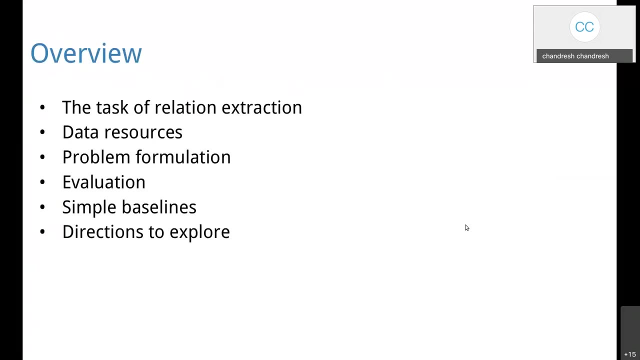 and let's say, supervised method and supervised method and so on, to solve this problem. okay, so, given this background, the problem statement, let us walk you through this one. okay, so we'll, throughout this talk, we'll understand what is the task of relation extraction, what are the data resources required to build a classifier for relation extraction. then we'll. 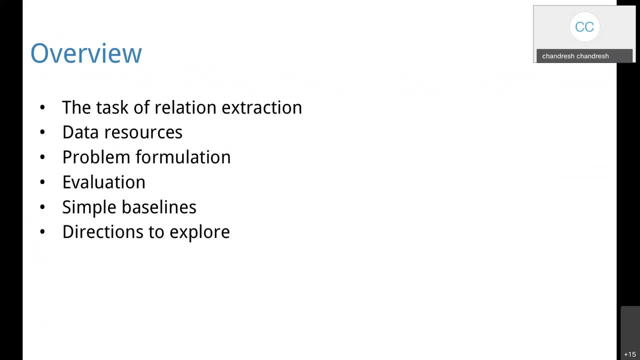 look at problem formulation, then evaluation and some baselines, right? actually, yeah, when I was started doing NLP then after this, very recently, I realized that relation extraction is very, very important in NLP compared to, let's say, just sentiment analysis. so once you have extracted the relation, it might be helpful in doing other tasks in NLP, such as machine translation. 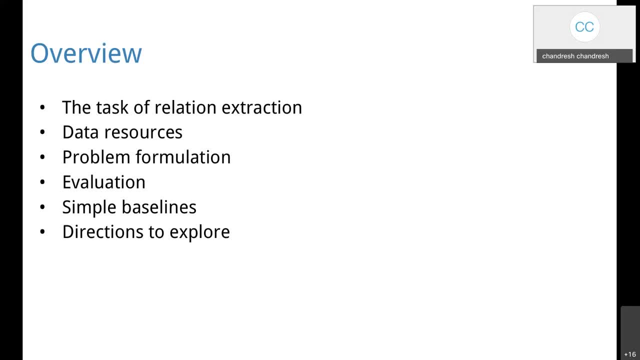 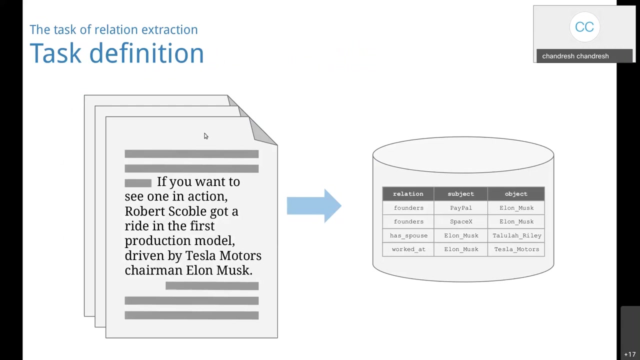 or semantic role labeling, or maybe sentiment analysis, emotion recognition and so on. okay, so let us understand the task of relation extraction will move from manual ways of extracting relation and then we'll go deeper and see how machine learning techniques can help us to solve this problem of relation extraction. right, so here is the task. let's say you are given a bunch of document. 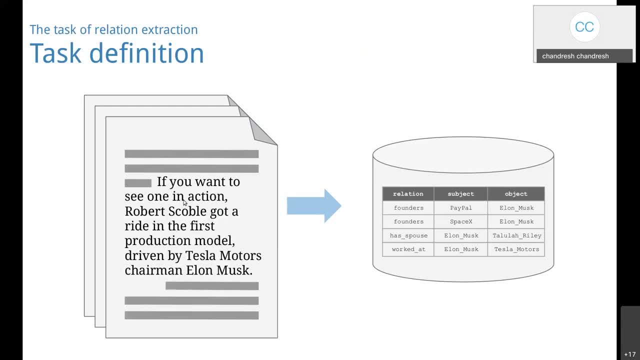 document here could be research paper, a news article or social media post. given this kind of corpus data, you want to to extract the triples. So relation is actually a triple of this format. So each row is a triple, where first column is a relation which holds between the subject and object. So, founder, 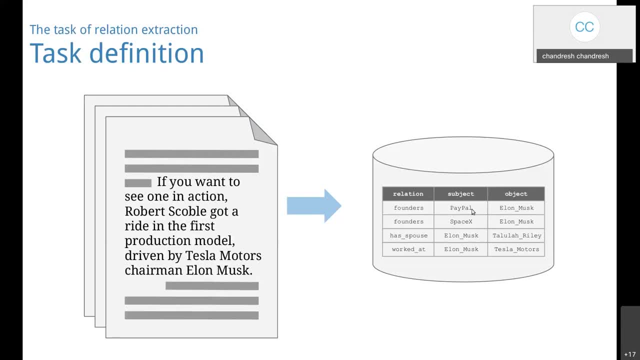 is a relation between the Elon Musk and the PayPal. So PayPal and Elon Musk are the entities and the founder is a relation between them. Similarly, founders is also a relation between SpaceX and Elon Musk, All right, And there are other relations which hold between Elon Musk and. 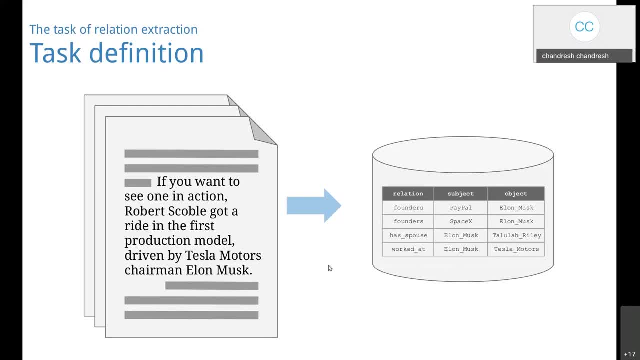 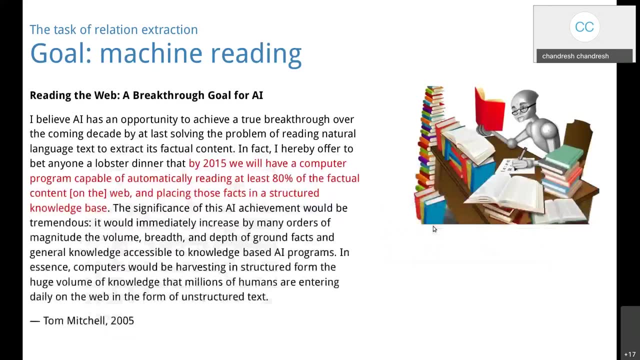 Tesla Motors and so on. So that's the kind of triple we want to extract from the corpus, All right, Okay, So the task of relation extraction, we want to do it automatically. So we want to resort to machine learning techniques. Okay, So I would skip this slide, I suppose. 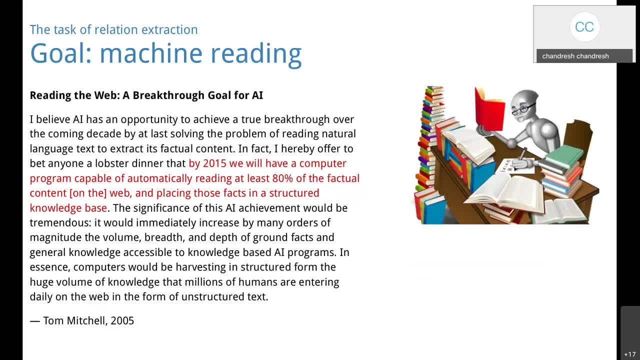 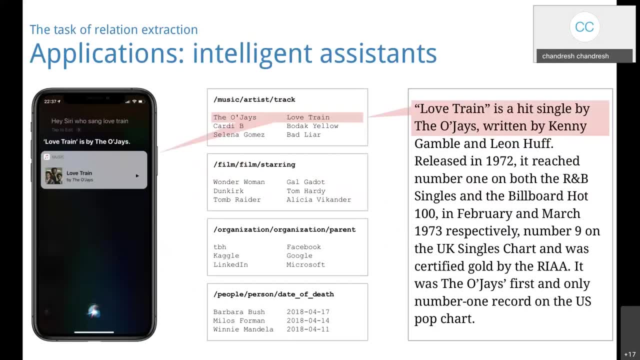 It's all about AI and how computer can be used to extract the relations Right. So this is what this slide is saying. So it has lots of application, as I mentioned, for example, here you can see that it finds application in intelligent assistant. So if you want to understand a track, music track- 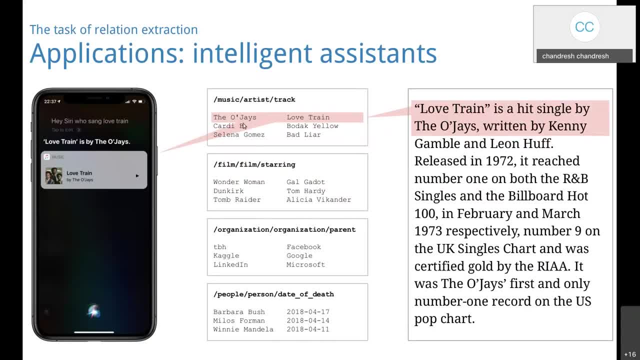 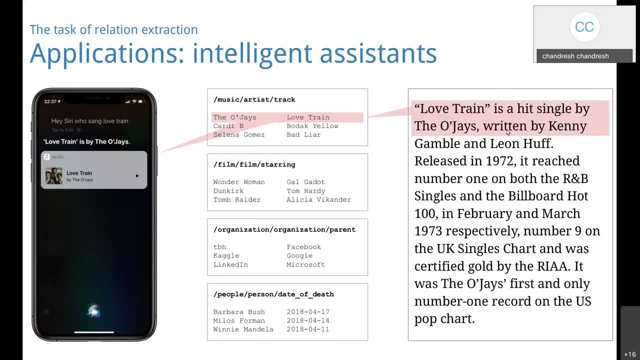 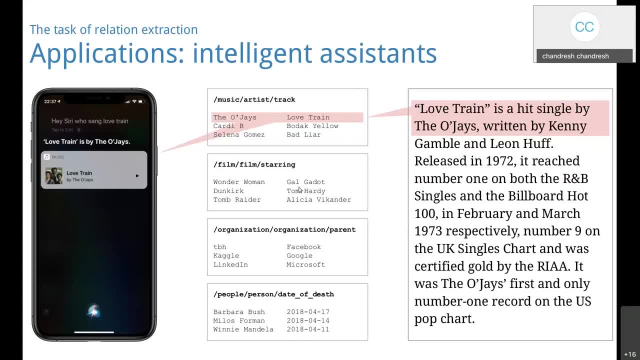 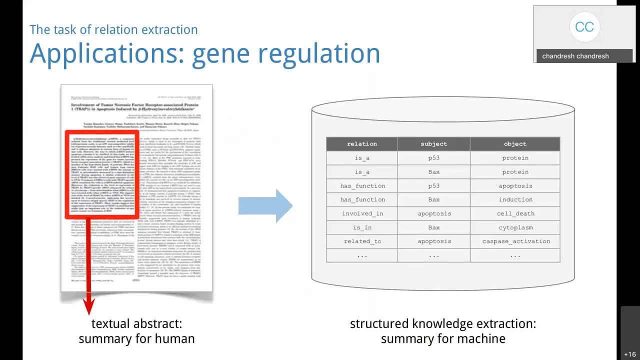 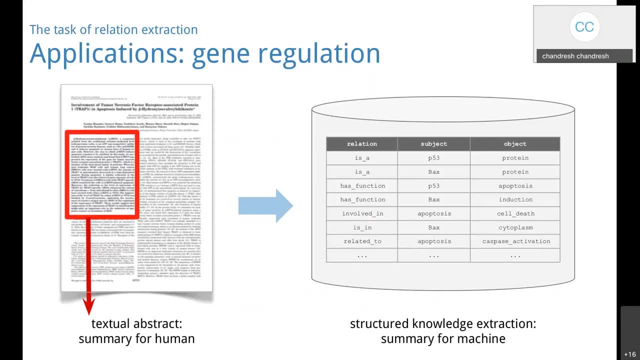 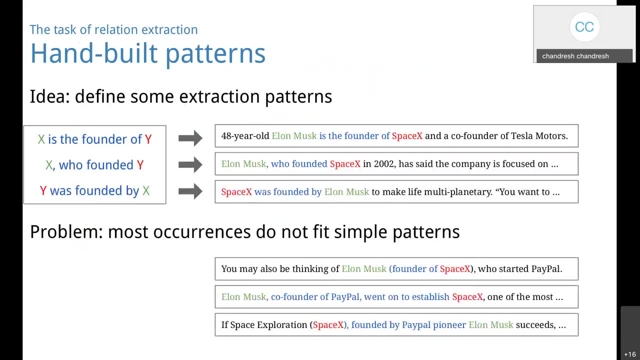 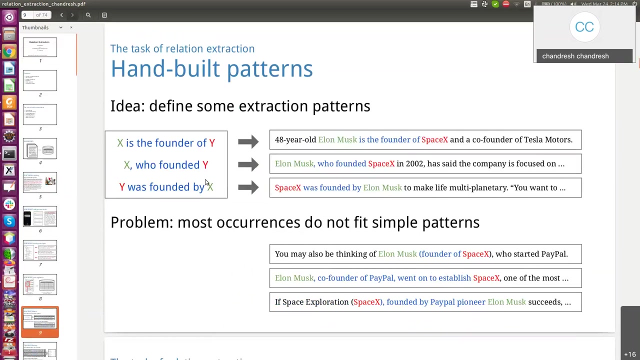 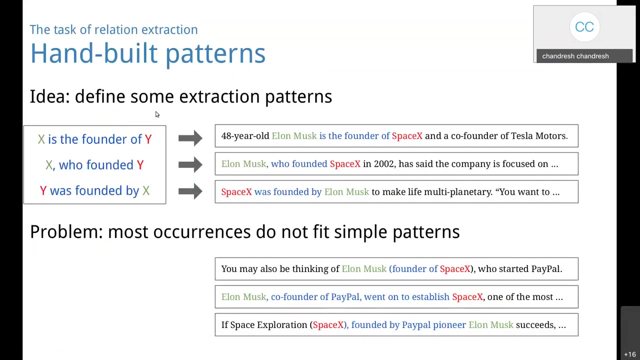 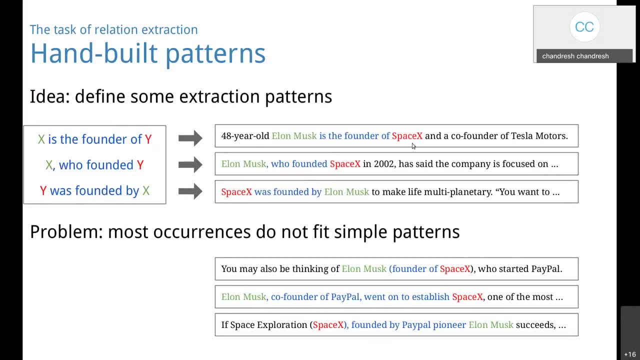 you replace x with elon musk and y with space x, so your reg x will extract this relation. elon musk is the founder of spacex, fine. similarly, if you write a rule like this, then you will extract relations of this kind. elon musk was founded spacex. who found it right? 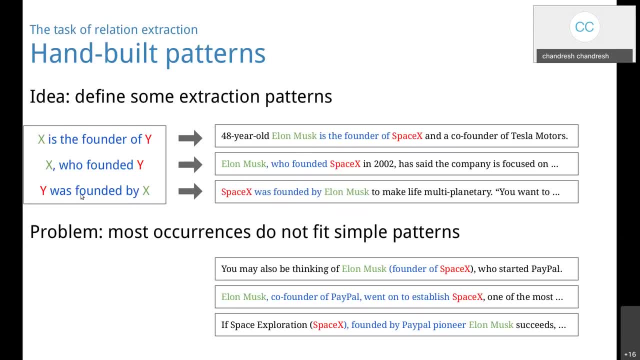 uh, but this kind of manually, you know, writing rules is not scalable. the reason is that if i slightly change uh, one character maybe, then this rule is not going to match the sentence right. for example here: if you look at this sentence, the same relation holds between elon. 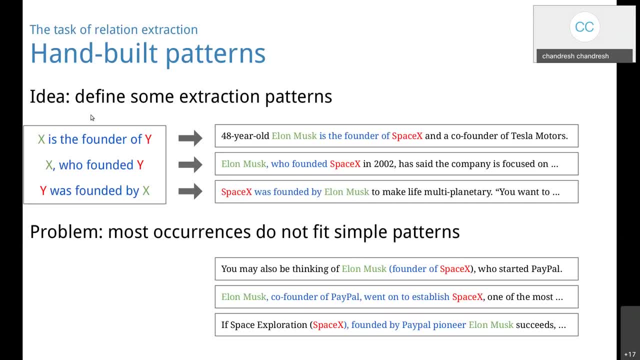 musk and the spacex, the founder relation. but these are the rules which you have written. they are not going to match with this sentence, right? can you see that? no, none of these rules is matching, so you'll miss these kind of sentences. that means there are false. 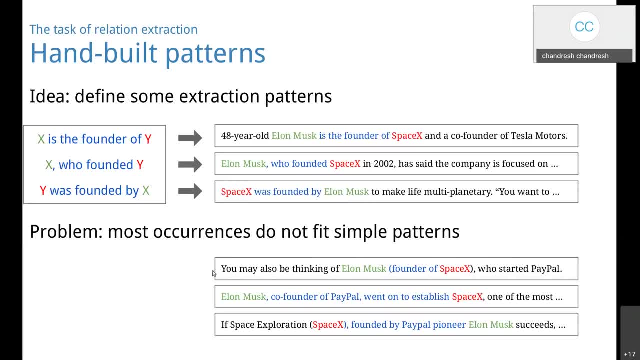 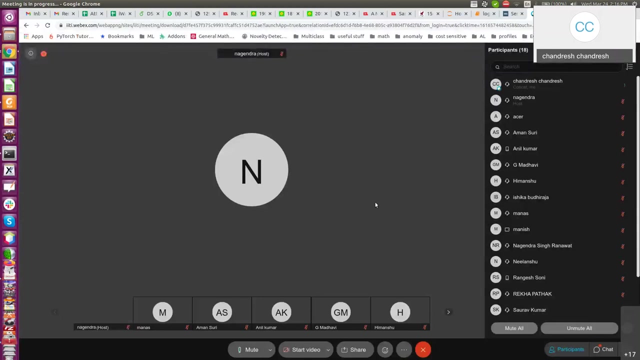 uh negative. oh yeah, so you are missing right. so you're, you are missing the true pattern, so your procedure will go down right. yes, so this is the problem. that means my uh reg x is not a scalable solution, so anyone has any idea what we can do to solve this problem? let me get some ideas from the audience. okay, so i hope the 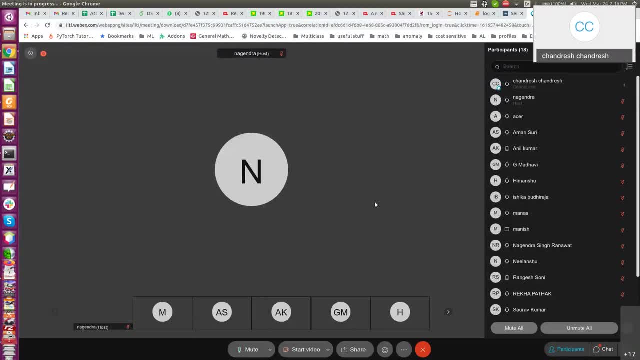 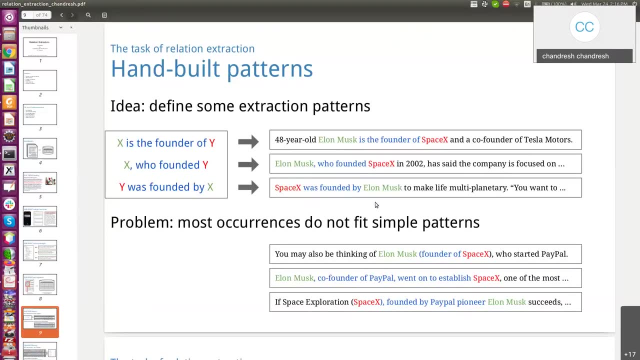 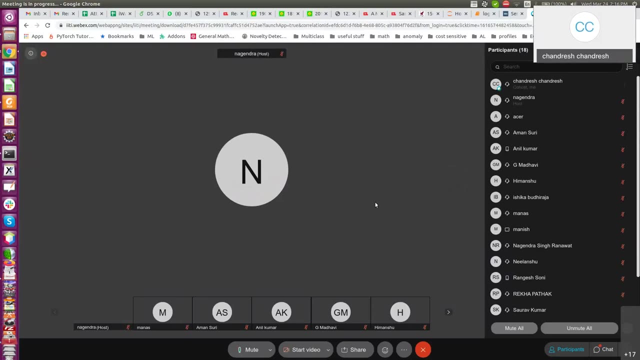 problem is clear, what we want to do. and let's say you want to solve this problem now. you don't have any prior experience, so let us get some ideas. what will you do as a data scientist? anyone throw your ideas sentence into two parts by the word founded and then search for the two entities that are required. 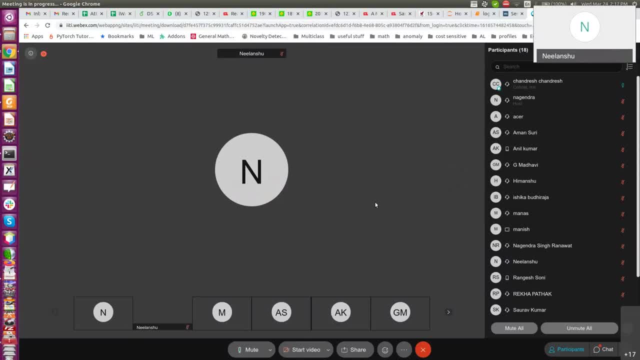 in the future. so you are saying that you will search for sentences containing the founded right? what? yes, okay, i see. then how would you identify the entities? there could be multiple entities in a sentence, right? so based on the occurrences, the number of time they occur, uh-huh, if we have. 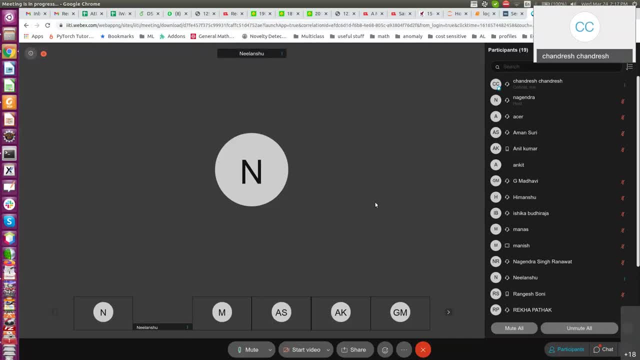 multiple data samples for the same entities, we can check the number of occurrences. okay, so you're going to go build a frequency based method, uh, where you want to extract the uh triples, right? anyone else has any other ideas? because in real life you encounter such problems where you don't know. 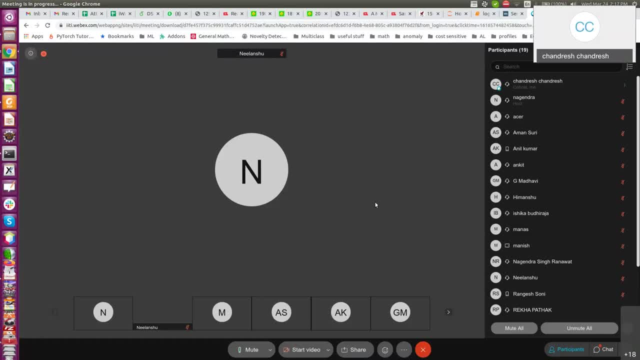 the solution. so you have to throw your own ideas right. himanshu, let us see himanshu, maybe can uh answer this query. if he's there or is she, can uh need not, you know, uh worry even if the idea you think is crap, that's fine, okay, but sometimes even 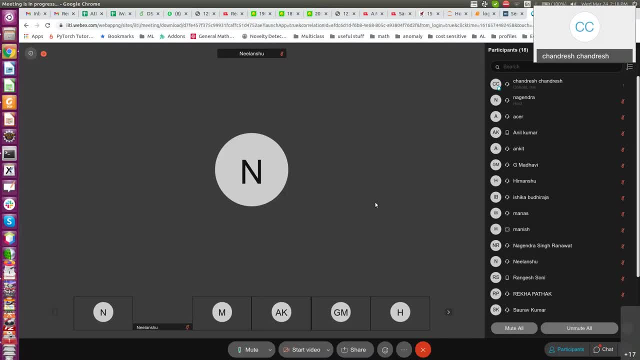 the. you know, uh, you start with a naive approach and you go with uh, with advanced solution, right. so now your approach is fine. so now your approach was, i think, uh, writing, you know rules, reg x, rules, and then trying to do this stuff right. so, can you, can you solve this? 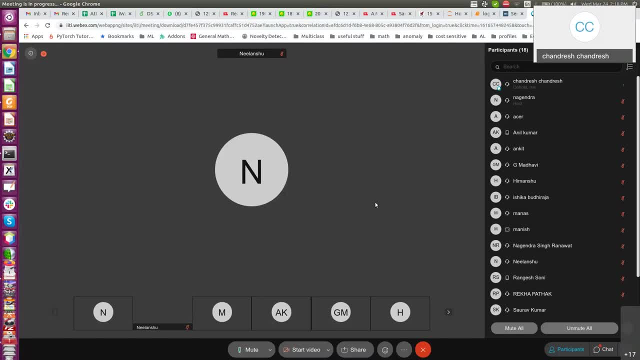 problem using supervised learning, because you have seen like supervised learning, unsupervised learning, reinforcement learning- you have been exposed to such kind of techniques, right? do you think? uh, here can we use a supervised learning method, anyone, in order to build a supervised classifier? what we need, what we will need: 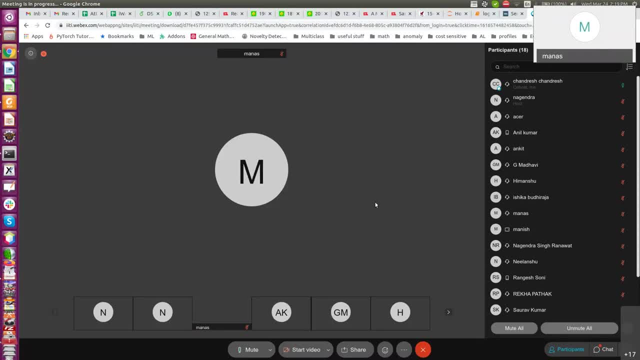 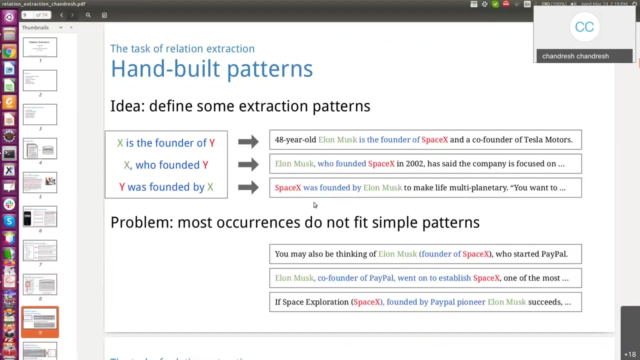 labels. uh, yeah, money, says amana says we'll need labels, right, so very good, what would be the features? the x1, x2, f3, the feature vector? right, we need that as well. right, to build a supervised classifier? yes, okay, yeah, yeah. so so yeah, we can usually try, uh, doing some supervised learning here. 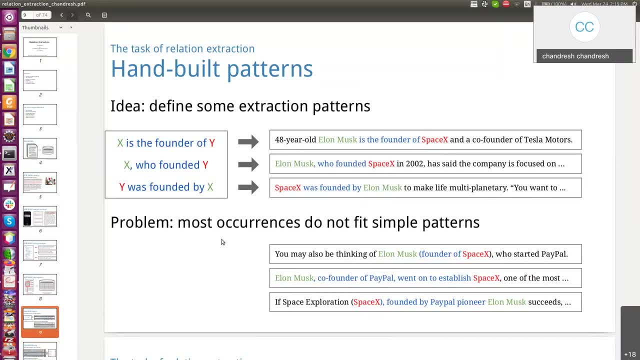 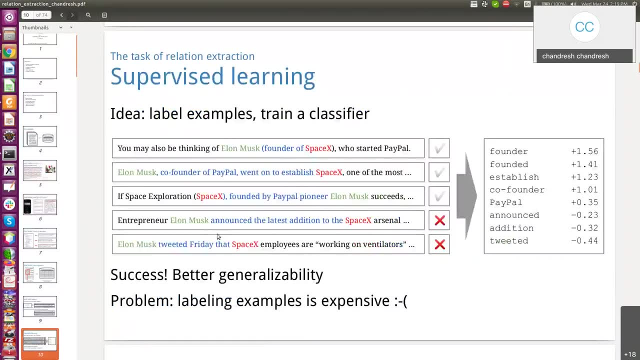 okay, so let me show you how we can do it using supervised learning, what would be the features and what would be the labels, and how to get the label. that's the most important. okay, so supervised learning, uh, so the idea is that label the examples, so you take the. 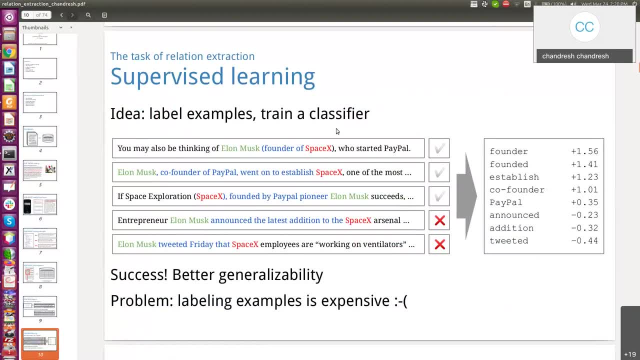 sentences and label them, okay, and then train a classifier. so here uh, here uh. let's say, if i give you this five sentence, you read this sentence, okay. let's say you are the annotator, uh, at amazon mechanical truck, which is a platform to get your data annotated. so you give the sentences to the 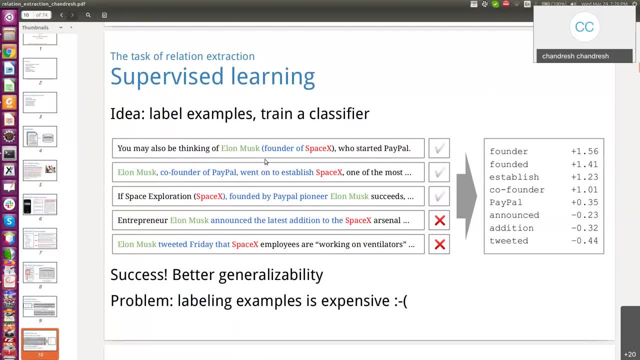 annotator and then they will say, okay, if there is a founder relation in this sentence, then i will put a tick mark. okay. and if you read the sentence, and elon musk and spacex, same entity, similar to first one, but founder relation is not there, right? 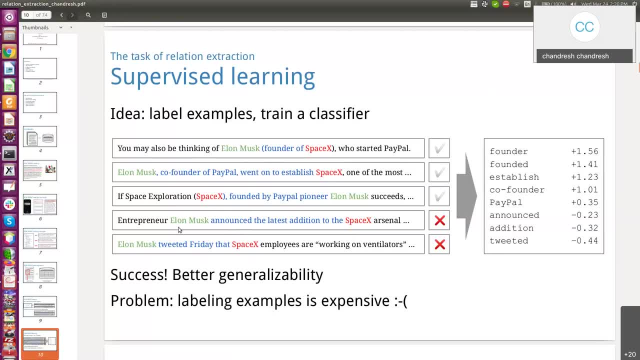 so if you read this sentence, it says that entrepreneur elon musk announced the latest addition to the spacex arsenal, right? so if you read the sentence, does it say that there is a founder relation? no, right? how many of you agree there is a founder relation or not in this one? 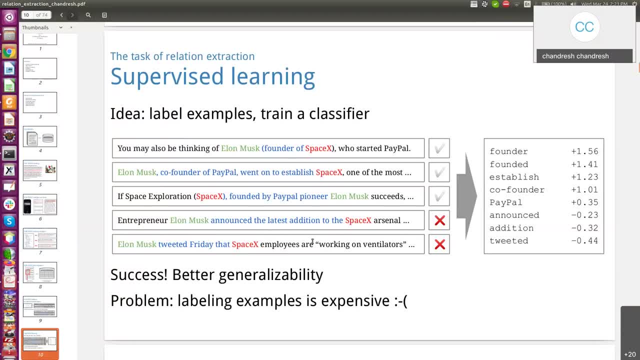 there is none right. so you put the cross right. that's how you label. so this is. it's like it's a plus one and these negative sentences are minus one. okay, and here, um, i think these numbers are saying the degree, how much? because in a sentence, 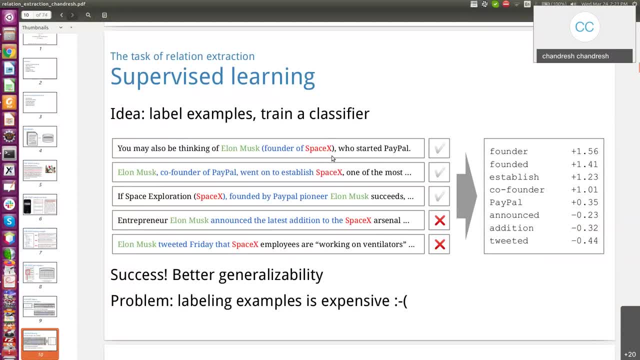 uh, when these annotators label the sentence, there you can also associate the degree of the relationship. for example, in the first sentence, the founder relation might hold with this much strength. okay, but because this is very subjective thing, some people might also say, based on their background knowledge: okay, lanmas is the founder of, let's say, spaces. they might also label this. 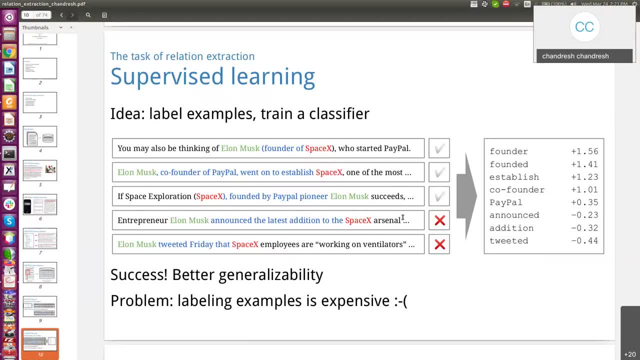 as a positive sentence if they don't know, uh, they don't understand the sentence completely, right? so this, these numbers tell you, uh, you know, uh, i guess positive, negative, they are saying the strength of the relation. okay, so you can take these sentences, build a feature. so your features would be: uh, you tokenize this sentence and 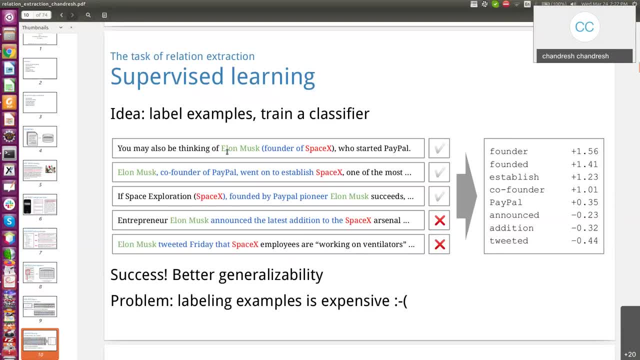 build. take a compute tf idea for the server to wake for your sentence, or compute sentence embedding and so on. so that's your feature vector x, and the label y is coming from here. okay, now you have your training data. you can split into train and test set. 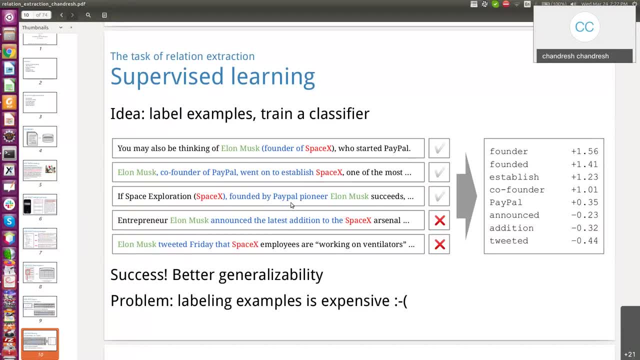 and then you can train any favorite classifier as via neural network decision tree, whatever you like. right, you can uh get some accuracy, that's fine. however, there's a catch here. the catch is that, uh, you need to read the entire corpus and label it with uh if there is a relation or there is no relation. so, 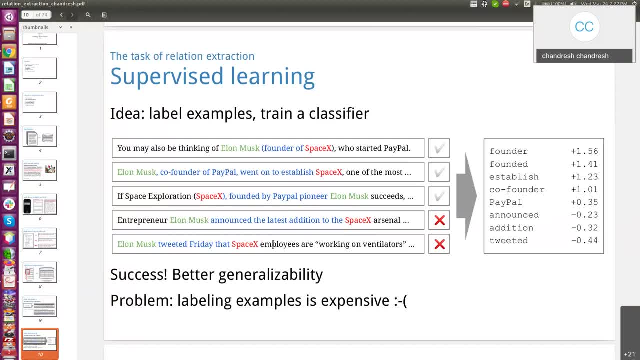 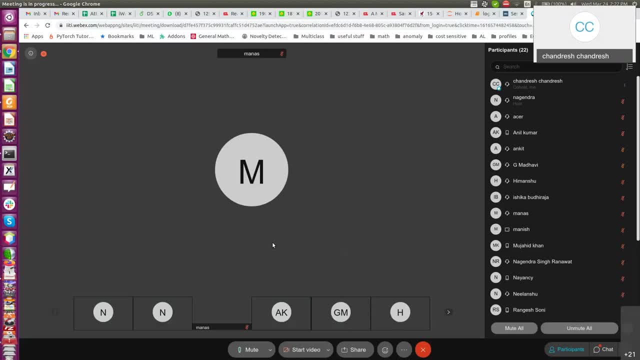 it's expensive, okay, getting the data annotated. in real life you get unlabeled data, okay. so whenever you, let's say, join a company tomorrow, so the client, the data they give you, is most of the time unlabeled okay, unless you are using benchmarks data set. so here the problem is that getting all your sentences labeled with relation or no relation. 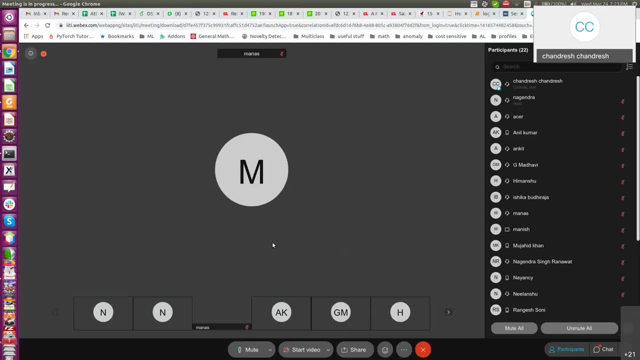 is expensive. so what to do? right? so anyone has any idea. if you can't annotate all the data, what to do? any thoughts? when you don't have lots of label data? what are the solution approaches? we can use musaid khan this year. manshi people are silent, very bad guys. throw some ideas so that we can talk about. yeah. 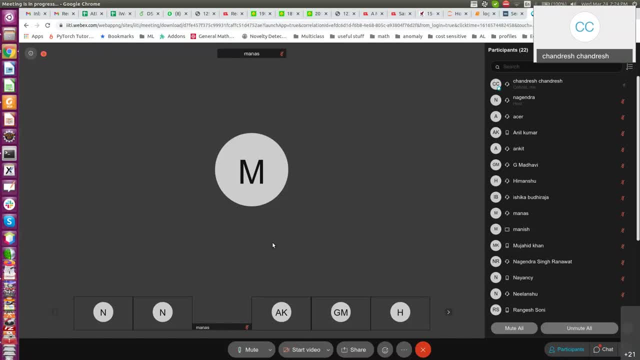 regression. we can nancy saying regression might help. why do you think regression can help? it's a classification problem, it's not a prediction problem, right? yes, sir, then how can regression help here? anybody is has any other ideas? okay, nobody. so if you already know the answer, then you won't be attending this talk, right? so 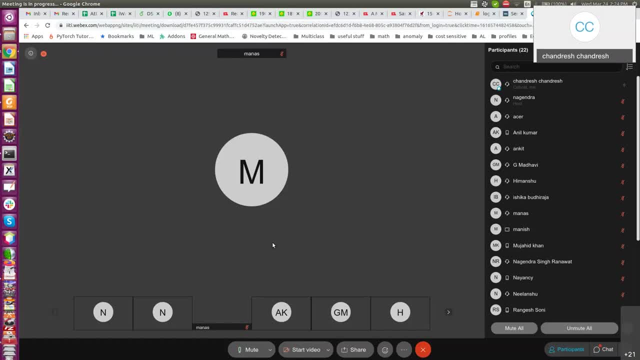 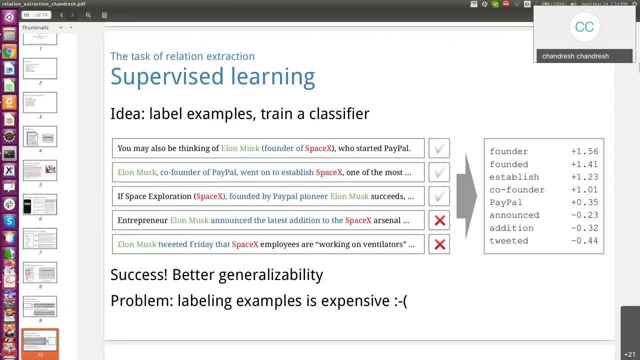 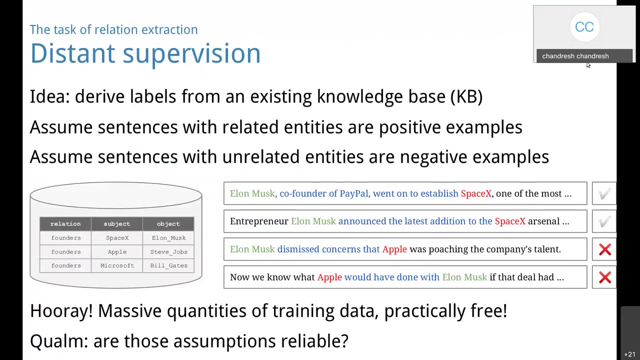 let's, let's see: uh, how can we solve this problem, right, when you don't have lots of label data, right? so? so the idea is to do a distant supervision when you don't have lots of label data. If somebody asks you- okay, I'm not going to give you lots of level data- then you can. 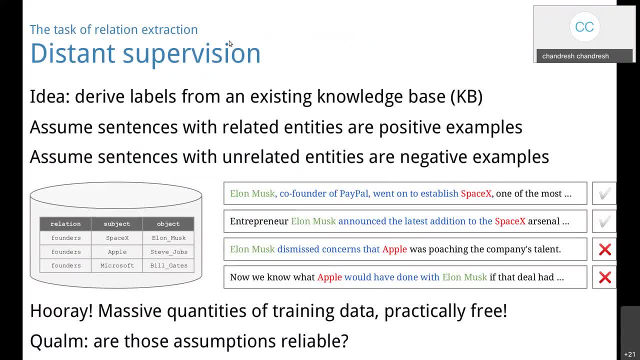 use such technique, known as distance supervision. It's a similar to transfer learning, where you train model on one domain and use it in another domain or fine tune it in another domain. Okay, so the distance supervision idea is like this. So first idea is that you derive the labels from an existing knowledge base, right? 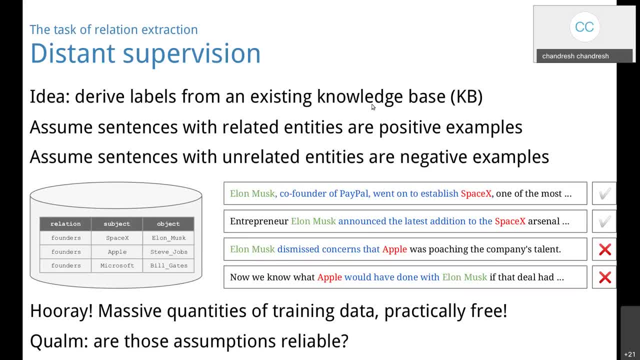 So what is a knowledge base? knowledge base is a collection of triples where you know the entity and the labels. for example, here is a knowledge base where you know that relation is there and entities are there is entities are space x and Elon Musk. okay, so you know. 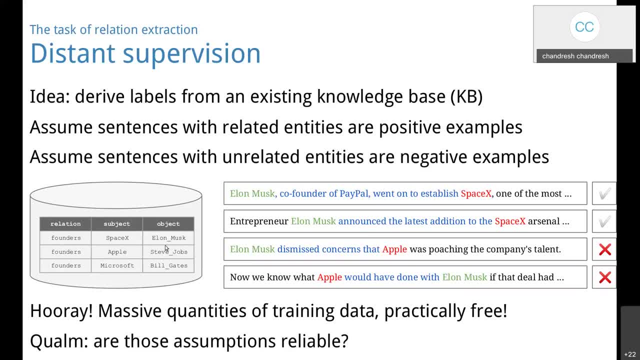 the relation. So this is a knowledge base that somebody has already curated in one domain. Okay, So this is what we want to make useful. All right, And so distance supervision means means you use labels from a different source. That's what this is saying. 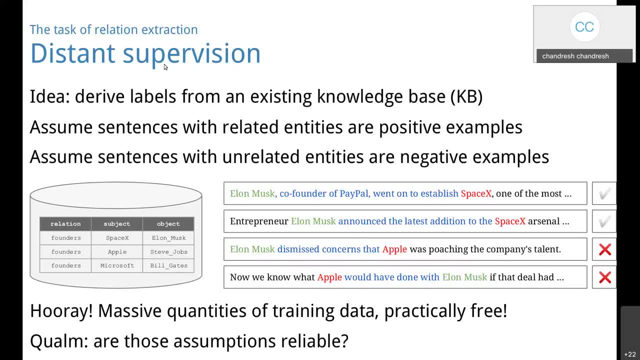 Distance supervision means you use labels from a different source, All right, And you also assume sentences with related entities are positive examples. For example: Ah, If a sentence In my corpus. So these are the sentences in my corpus that I want to get labels for. 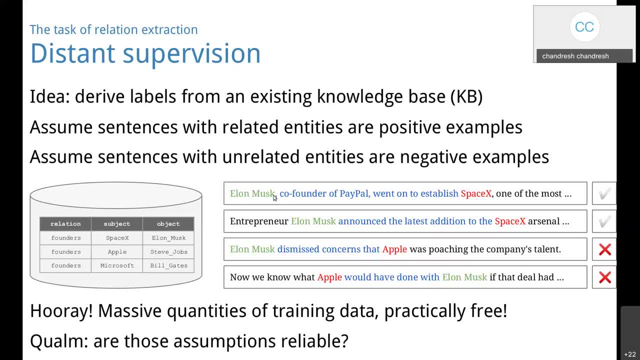 Okay, So if I read first sentence and see if the two entities are present, for example enormous and SpaceX, I will search these entities in my KB and if I can find these entities and then I will mark as a positive example or there is a relation so Elon Musk and SpaceX. 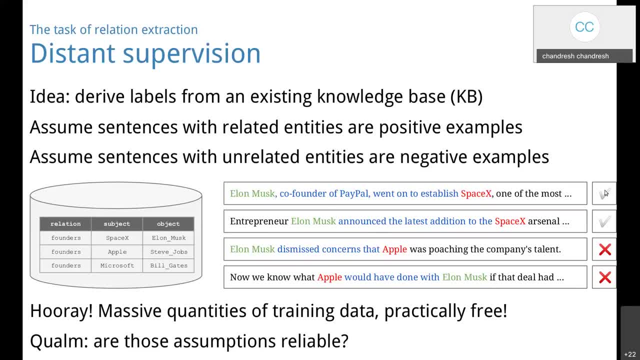 are there. So I will, I will say tick mark, Okay, Right, tick mark. And if you, similarly, there is a Elon Musk and SpaceX, So you again say right, tick mark. But if you look at this one- Elon Musk and Apple- we search for these entity pair in our 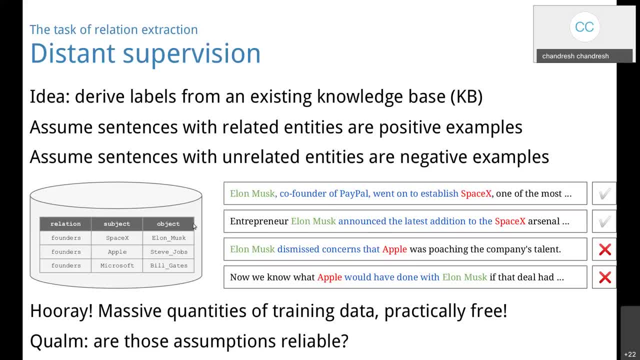 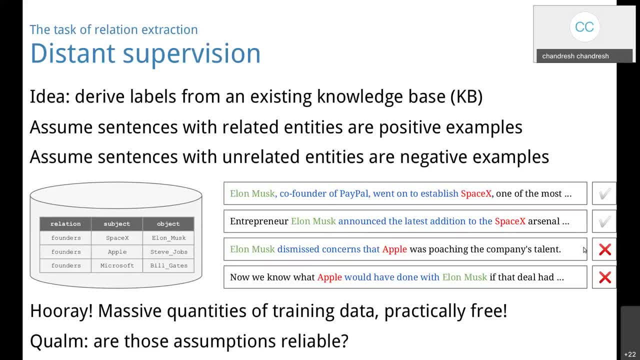 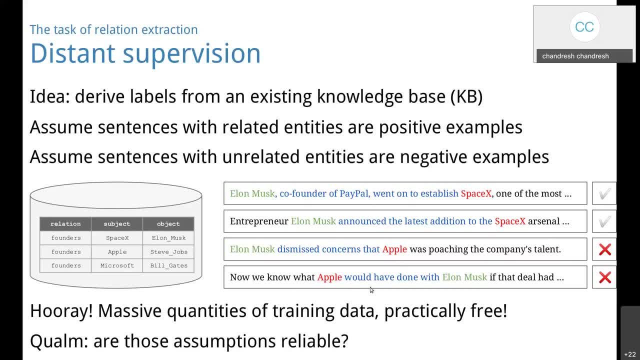 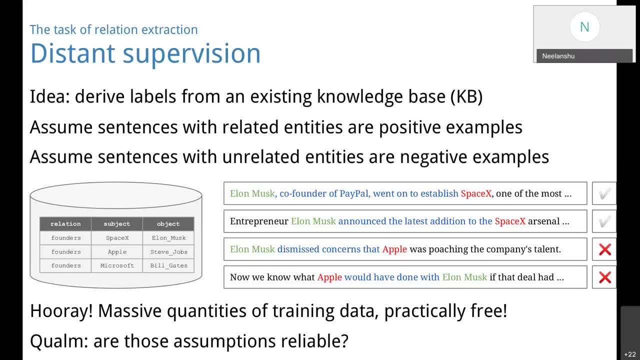 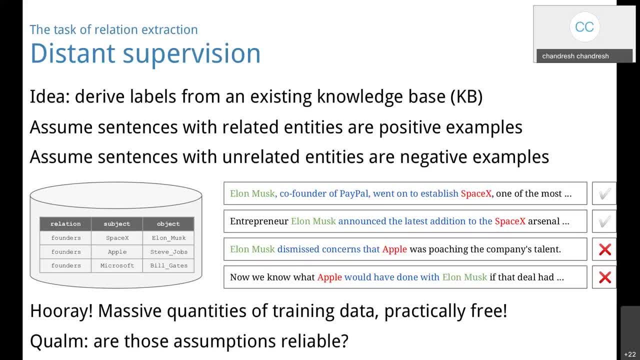 So in machine learning on an LP or information retrieval, there is a whole field that we call knowledge base completion, KB completion, in which we try to fill all the possible entities pair in the domain. Okay, So there may be entity pair which is here and there is a relation, but that entity is not present in KB. 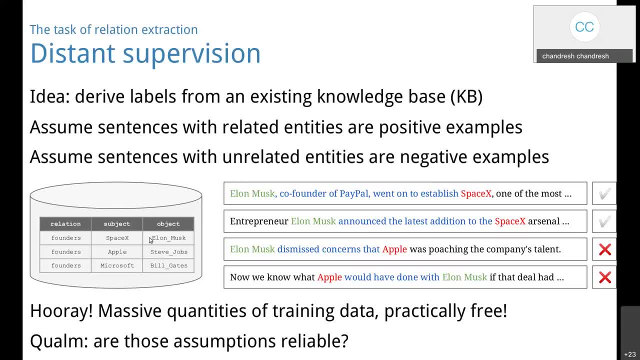 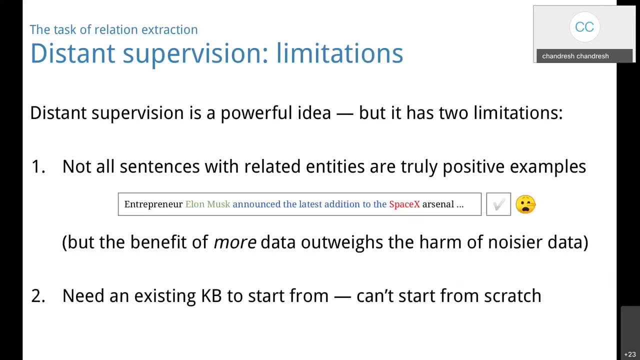 Then that's bad. Okay, So there could be vice versa also. Right, And there is a, for example, entity pair, but there is no sentence, So you're not going to use that, but that's fine, Okay. So yeah, distance supervision is a powerful idea, but it has two limitations. For example, not all sentences with related entities are truly positive. Okay. 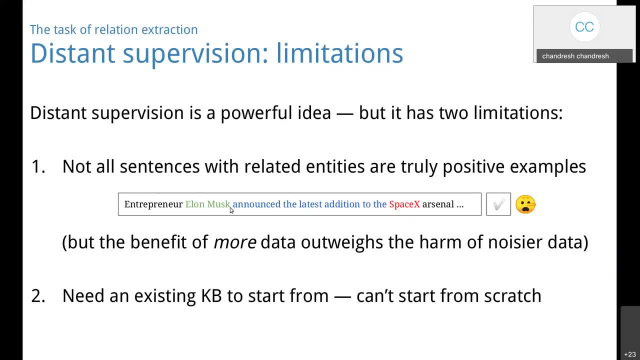 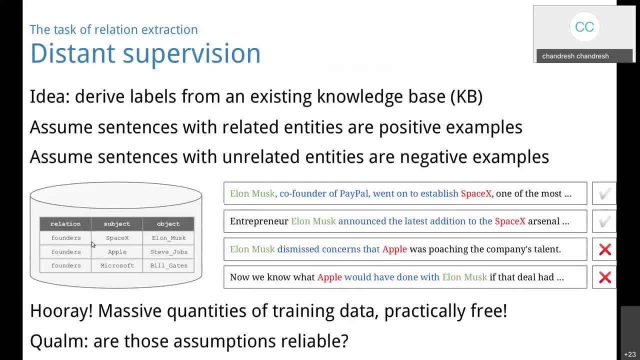 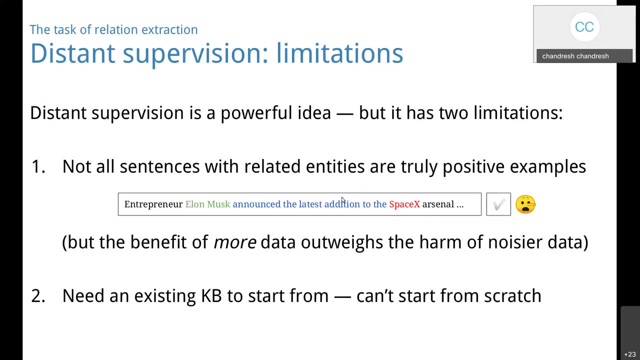 For example this sentence: that entity pair is present in landmass and SpaceX. This entity is present here. Then you will say: quickly go ahead and label it positive. Okay, But if you read the sentence, does it indicate that there is a founder relation? Right, Read the sentence and tell me if there is a founder relation. Is there? 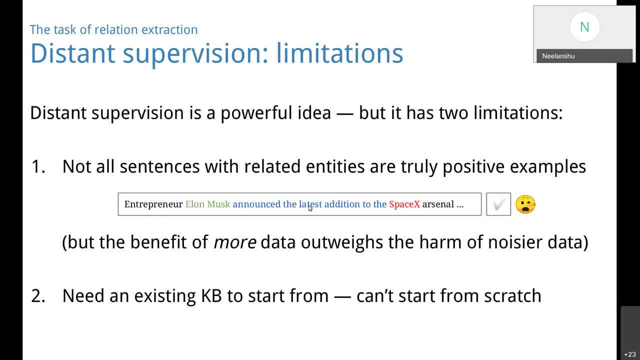 No, sir, Entrepreneur landmass announced: Right, There is no founder relation. So that's bad. So you are labeling Same, labeling the sentence in a wrong way, Yes, So that's a bad idea. So what is happening here is that you are adding the noise, Okay, But, as you will see that, the benefit of more data. more data how? because you are labeling all the references, right. 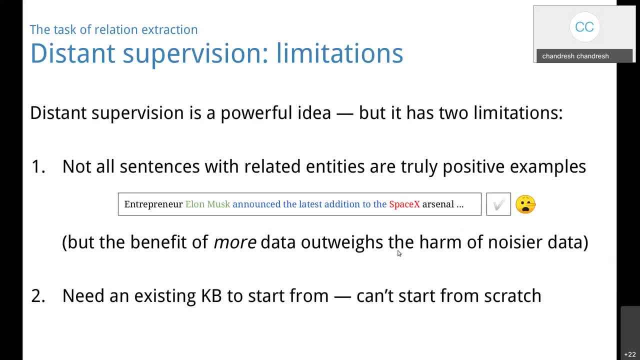 So the benefit of more data outweighs the harm of the noisier data, Right? So this is actually nice, But such kind of noise you can expect. they are very less, maybe 1% or less. Okay, So you can safely assume. 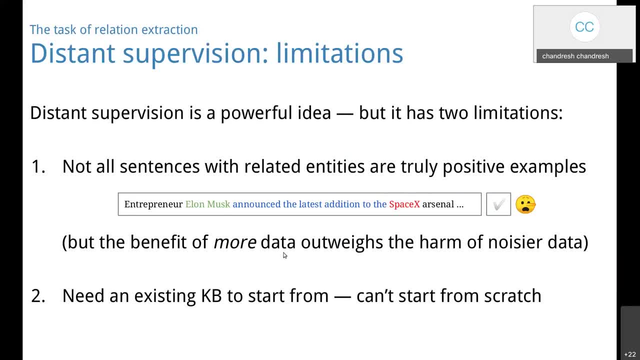 that, uh, you know, the noise is very less and you are getting more training data, so fine, uh. second problem here is: need an existing kb to start from, so you can't start from scratch. so if you don't have a kb in your domain, then you can't do this thing. all right, so that's. 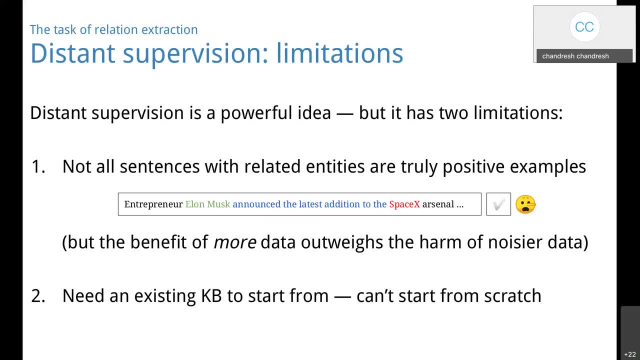 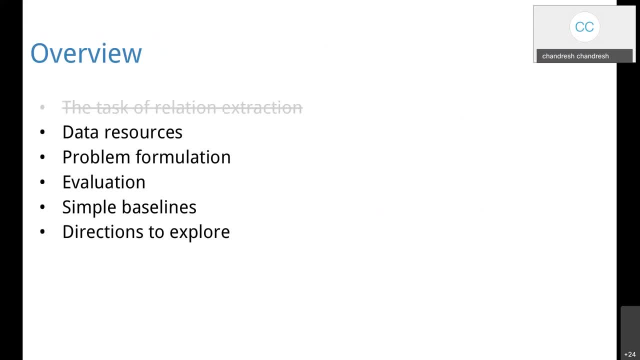 another limitation, because not all domains have their kb right. uh, okay, so, having understood the task of relation extraction, let's see what are the data sources where we can hinge upon our solution, and then we see solution approach. okay, so the data resources that we are going to leverage: uh, 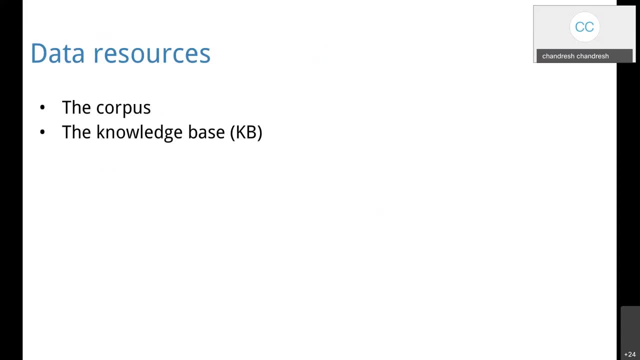 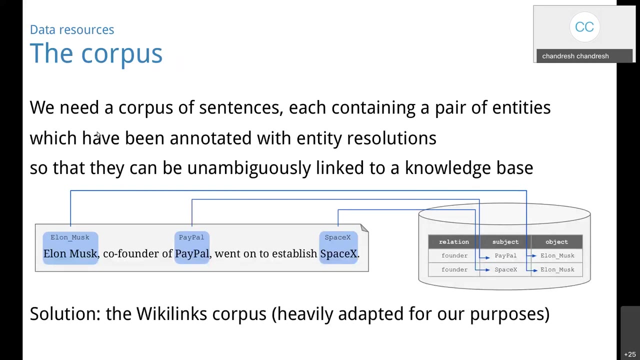 first one is the corpus and second one is the knowledge base. okay, we have already seen both of them. the idea is that to connect these two together, okay, so let's see. let's see what is our corpus. so we need a corpus of sentences, each containing a pair of entities. so this is a corpus. right, you can think. 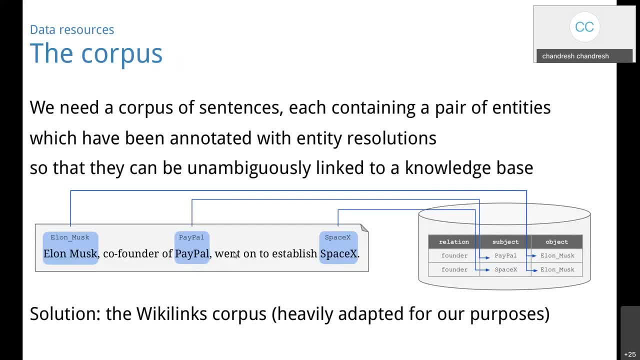 of one sentence is one corpus and this corpus are sentenced as a entity pair and this entity pair have been annotated using a knowledge base. can you see that in a mass paypal? okay, there is these two entity pair and relation is founder. okay, and the idea is that the way these entities have been 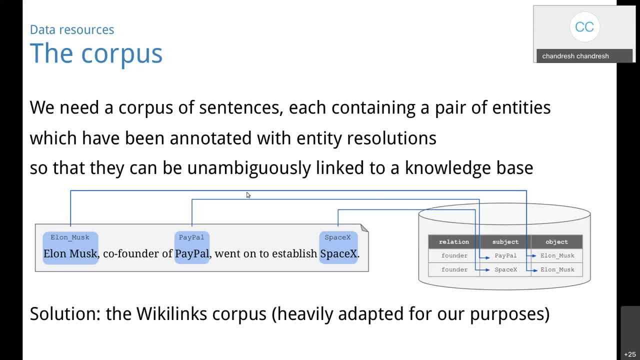 related using this kb. they must be unambiguous. okay, they should not be ambiguous. so actually ambiguity is a big problem in nlp, because same word can mean different things, right? for example, new york's. if there is a word new york, so new york can mean new york state or new york city. 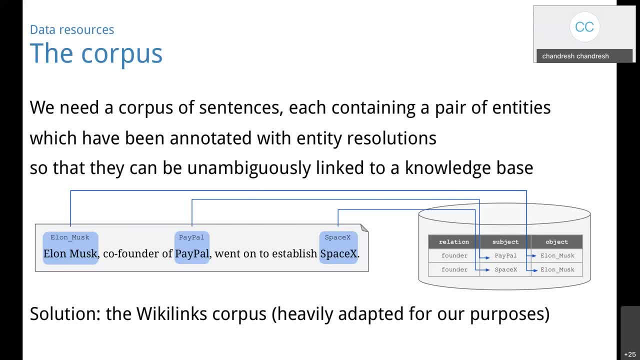 similarly, uh, there's a bank, right, so bank might refer to the river bank or financial entity, right. so we assume that, uh, this kind of thing uh has been resolved, uh, and there is no ambiguity in the knowledge base, otherwise you would be in problem. okay, so yeah, so, uh, the wiki link corpus is a huge. 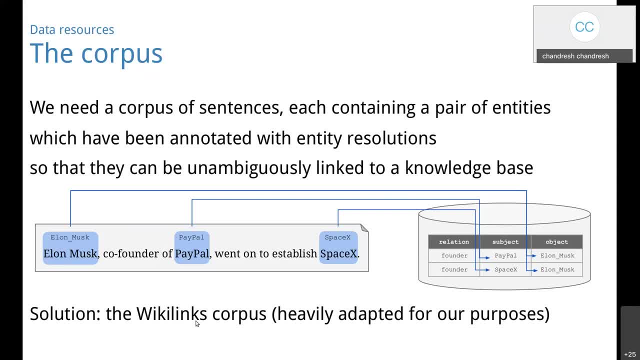 corpus collected by google's, and this corpus uh contains the entities, million entities, three million- i guess three million entities are there, collected by crawling 10 million web pages from wikipedia. okay, so google has lots of data. so the nowadays, uh, in our olden time, right, we had 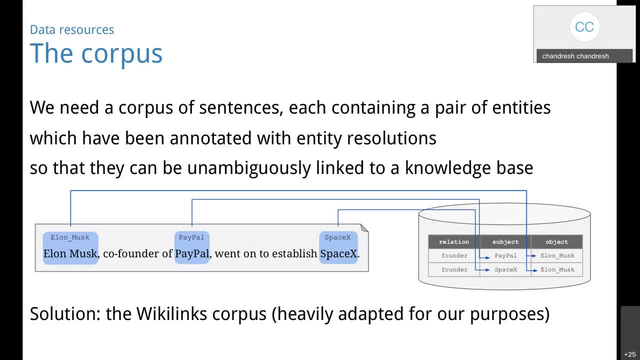 our stone age, and then i guess: uh, which other age was there, right? uh, after that, maybe cool age was there. after that we have, uh, 21st and 22nd century data age. okay, so that the more data you have, the more powerful you are, okay, so, yeah, so the way the 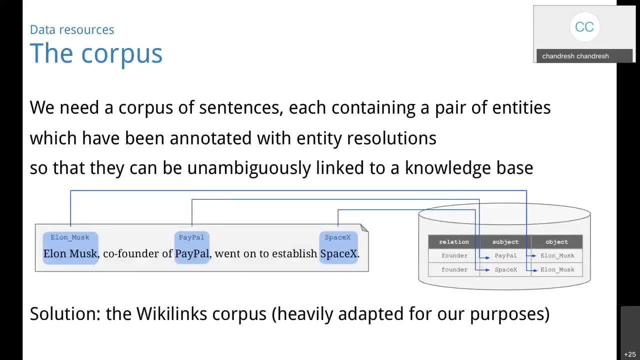 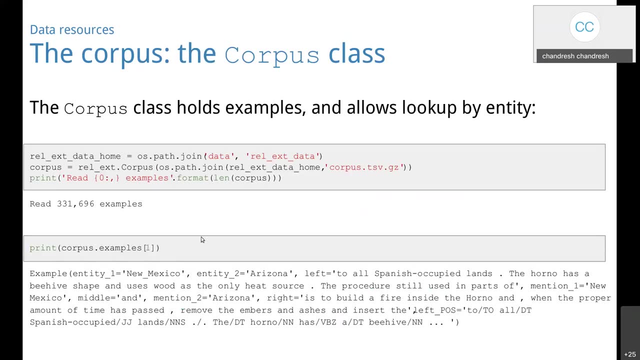 corpus. so in order to so this, uh, this talk is more focused toward how to do actually relation extraction. so let us go in uh, do deeper and see the code actually how it is done. so, uh, maybe i share this one also at the end of the workshop. so we have this corpus class uh, which is there, okay? 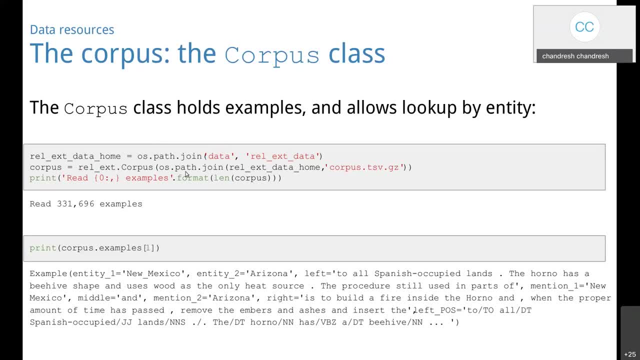 so the code, i will say there is a corpus class, so it has actually all this corpus data, right? so in this corpus we have these sentences. so total, in our corpus there are around 300 000 sentences. uh, for example, right, and if you look at one of the example you have these entities, okay, so first, 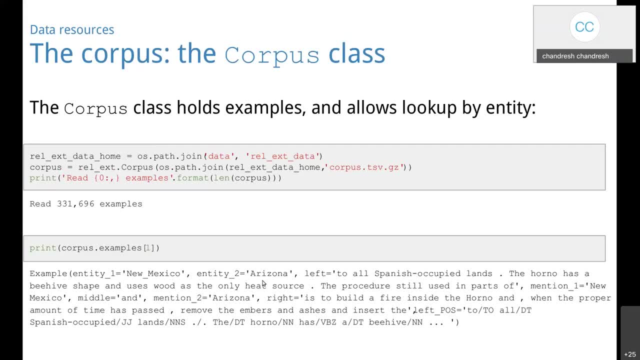 entity is new mexico. second entity is arizona, and there is a left. left means all the words which appear to the left of the first entity. okay, so this, actually this is a hold, your sentence or paragraph, and you have just split into two which, which is the first entity, which is the second entity. what have? what appears on the left. 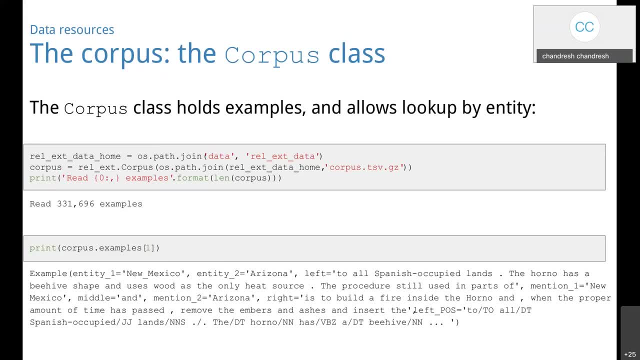 side of the first entity, what appears in the middle of the two entities, and so on. right, so this is just a split of your sentence. all right, entities were made manually in this example. uh, no, no, this. this data corpus has been compiled and, uh, they have been marked and this is entity one. this 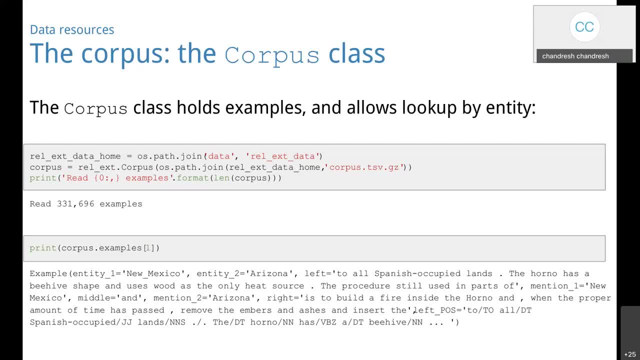 is entity two. okay, so otherwise, if you don't have entities already marked, you can run named entity recognition ner. there's a tool, uh, available in a scikit or nltk you can use, or stanford ner you can run to extract these entities. okay, um, yeah, so entity are very important in nlp, right? so entities are basically. 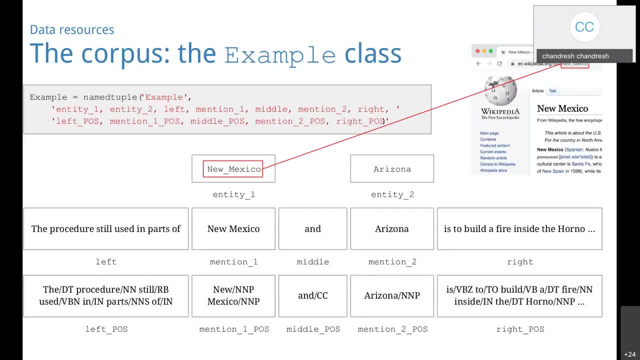 your noun phrases you can think of: so, yeah, so if you look at the corpus example class, okay, so you will see that uh, first entity is basically referring. for example, if the entity is named like this: new mexico, here can you see new mexico, new underscore mexico. this basically comes from the url of a wikipedia page for new. 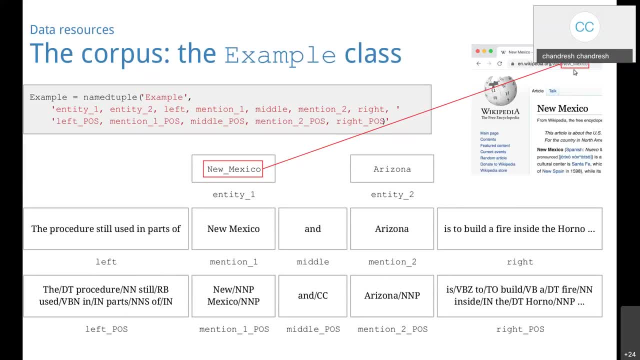 mexico, right. so if you open new mexico web page, wikipedia, then the last string in the url is that url is basically first entity, okay, and this other steps come from the page, this wikipedia page. okay, so if you check, maybe new mexico, if the page is not updated, you will see. 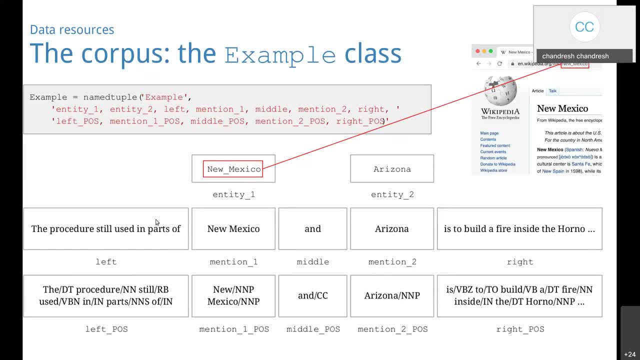 the sentence is there, okay, and if you combine so, left is this one, mention one is the first entity, mention two is the second entity and is the middle, okay, middle, and then there is a right comes after the mention two, then left. pos is a part of a speech, of this whole thing. 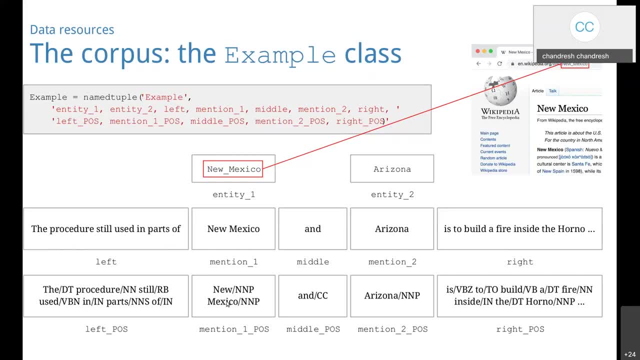 mention one part of what is the part of the speech of the first mention. mexico is, for example, nnp, and then p is a noun phrase- okay, and it's a coordinating conjunction, and arizona is again a noun phrase and the part of the speech of the right sentence. so this is: 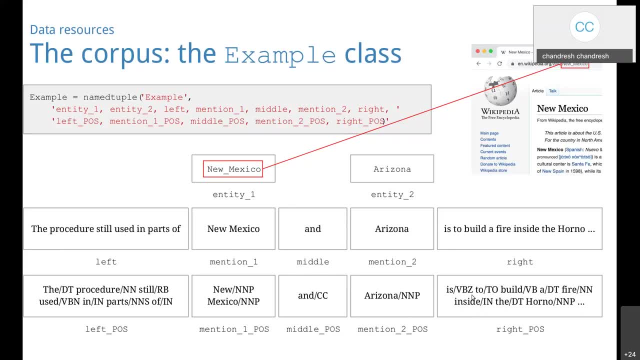 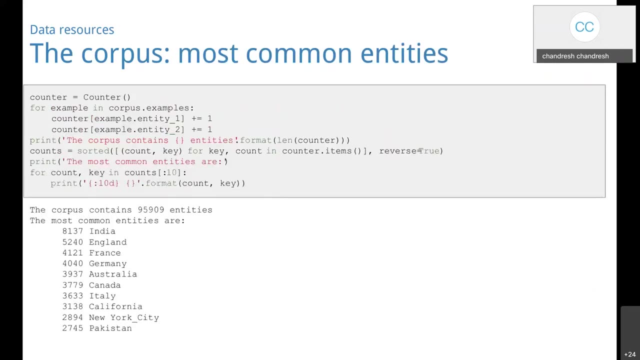 just, uh, you know part of the speech, of the sentences or the phrases, right? so this class, if you use directly, can poke around the sentence and it will tell you all this thing: entity 1, entity 2, and so on. so this is a compile data, okay, uh, so if you look at your corpus, 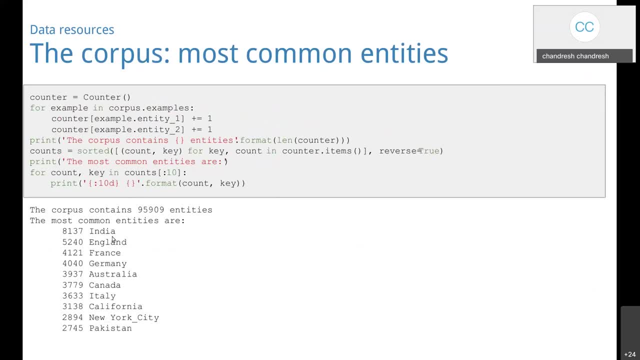 all right. so this corpus has uh total 95 000 entities in total, and the most common entities are basically, especially the country name- india appears up to come first 80 100 sentences, uh england, followed by then france and germany. so these are the entities. 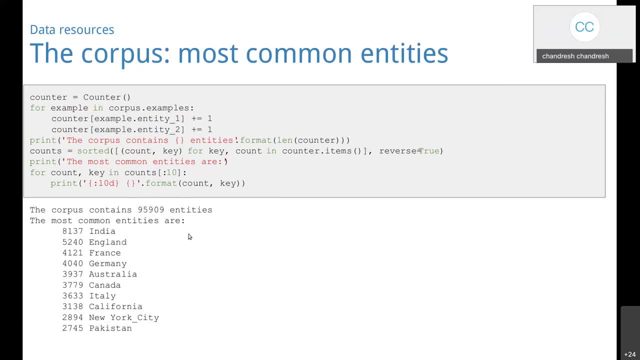 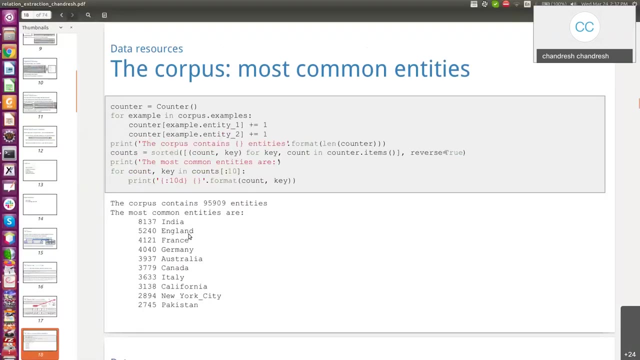 and this is the frequency of these entities present in the corpus. okay, um, i hope people are following. yes, um, anyone here lost? let me, it's very simple, just uh. if you focus, okay, if you want to learn something seriously, then you have to pay attention to right. so it's. 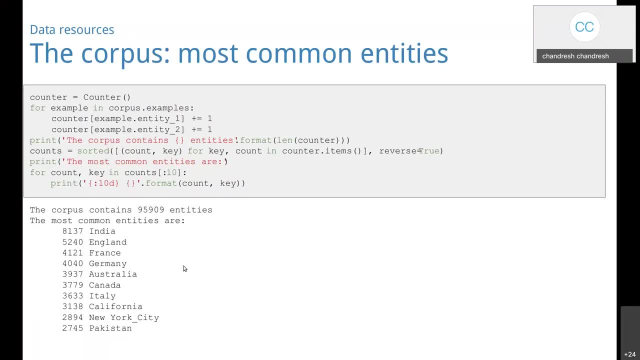 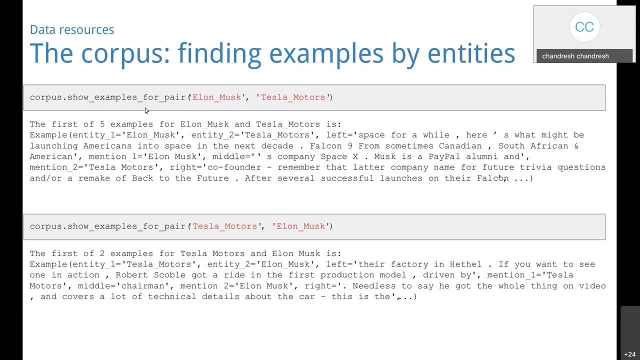 just a corpus class, uh, and we are trying to understand what is there in that corpus, right? so we are trying to understand how many entities are there, what is the frequency and so on. um, yeah, so if you further look around your corpus class and look for the examples of pairs, 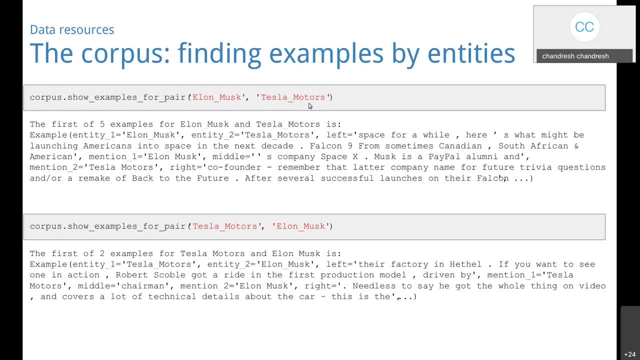 for example, you want to see elon musk and tesla motors, so how many sentences are there which contain these two entities? so it will tell you: total five sentences are there which contain these two entities: elon musk and tesla motor. one of the example is this one. okay, 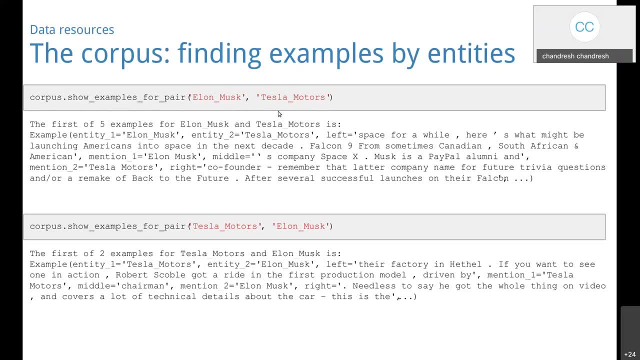 and if you just reverse the entity, make tesla motor as first entity, elon musk as the second entity, then you see there are only two examples which have this, these two entity in this direction. okay, so here direction is very important. for example, if i say: narendra modi is prime minister of india, now if you reverse subject and object, 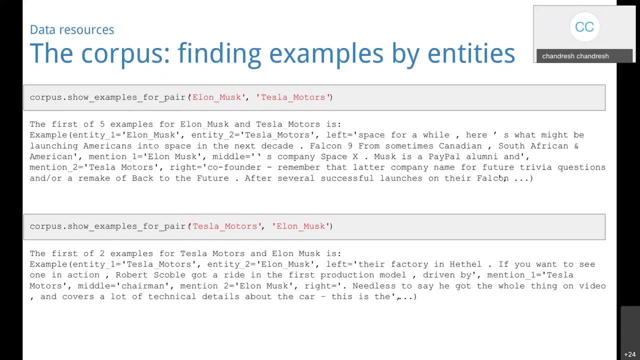 what will happen, right, so same relation might not hold. for example, india is not prime minister of narendra modi, right? so sometime relation hold in one direction, sometime relation might hold in both the direction. okay, for example, elon musk founded tesla motor, so founded is a relation, okay. but if 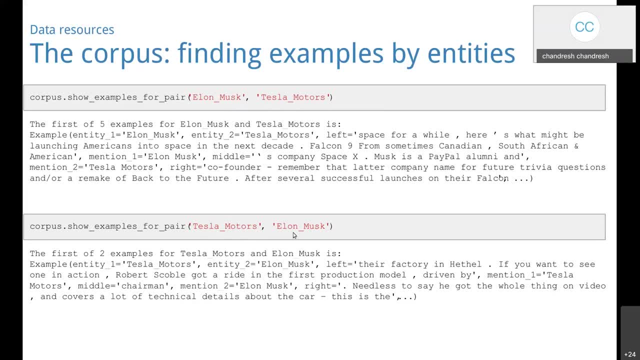 you say other tesla motor. you know, elon musk, that's not true. but there may be other relation, for example tesla motor, uh, you know, uh, here let's let's see if relation is there. relation would not be there actually in this corpus, only entity mentions would be there. so you can say tesla motor is established. 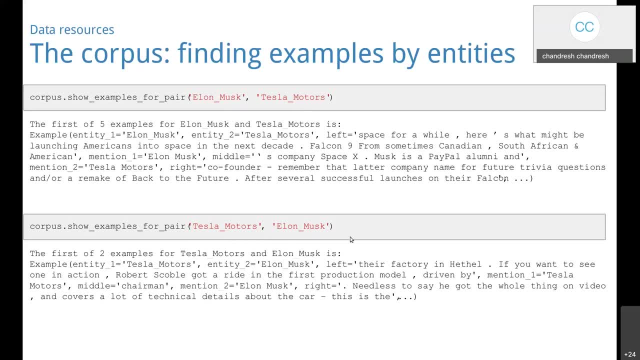 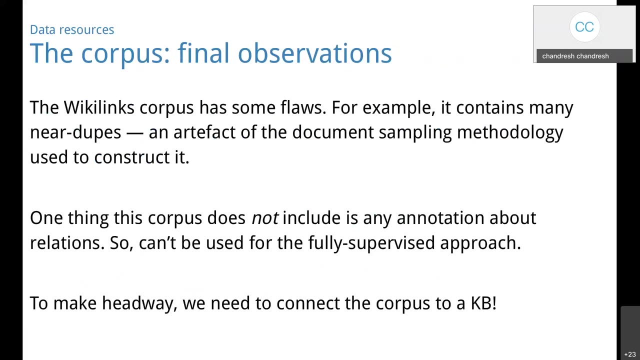 by elon musk, maybe. so establish another relation, okay, yeah. so yeah, see, in one direction, uh, one relation might hold. sometimes, uh relation might hold in both the direction, right, so we'll see an example quickly. so what is happening in our corpus is this: uh, so corpus is uh collected from wiki links, okay, and wiki link corpus has some flaws. 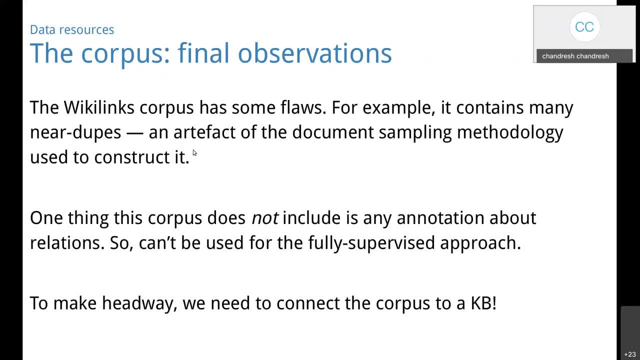 for example, it contains many near duplicates and artifact of the document sampling methodology used to construct it. so there are some newer duplicate, uh. another one is uh. one thing this corporate doesn't include is any annotation about the relation, so can't be used for the fully supervised approach. can you see that if you look at this? 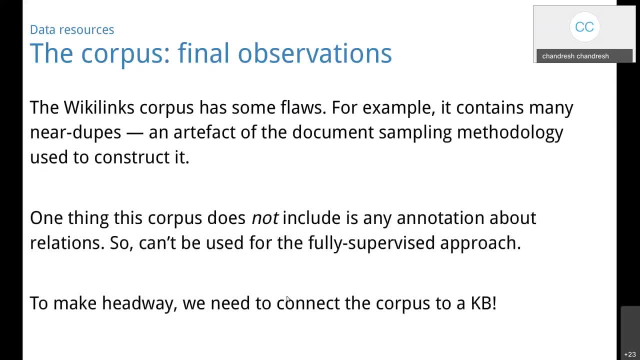 sentence there is no relation mentioned, right, so there is no relation. so you can't use fully supervised approach. so in order to solve your problem of you know, annotating this corpus, you need to connect this corpus with your kb. all right, so knowledge base, i'm going to 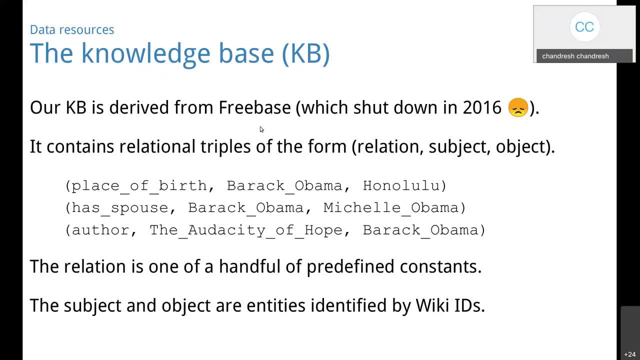 explain: uh knowledge base is derived from a freebase. uh, freebase actually was a project uh started uh uh, i think, out of stanford park or maybe google, so it had lots of actually triples of these entity pair and the relationship between them. so it has this relation. subject: 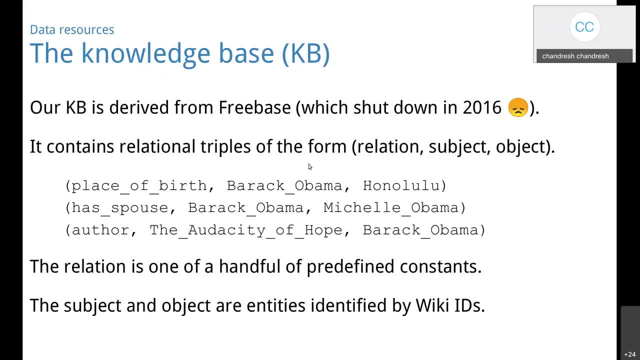 and object. however, it has been shut down now, but you can still get freebase uh download freely downloaded, downloadable from some sources, and it's a very good tool and it's very easy to use. it's a very good tool and it's very easy to use. it's a very good tool and it's. 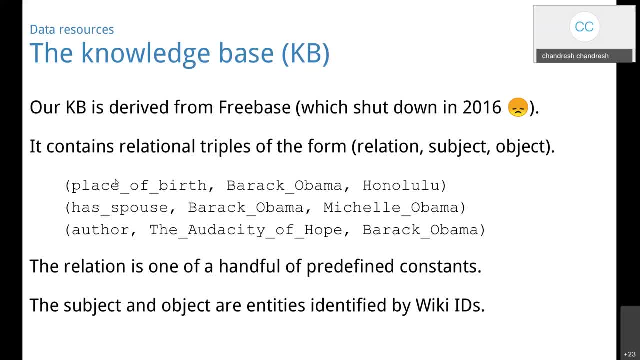 so it has this, you know, triples. right now we want to make use of these triples to annotate the relation in the corpus that we have from wikileaks, right, uh. so the thing is that, uh, this is a small kb total number of uh these relations, so relation we will be using as: 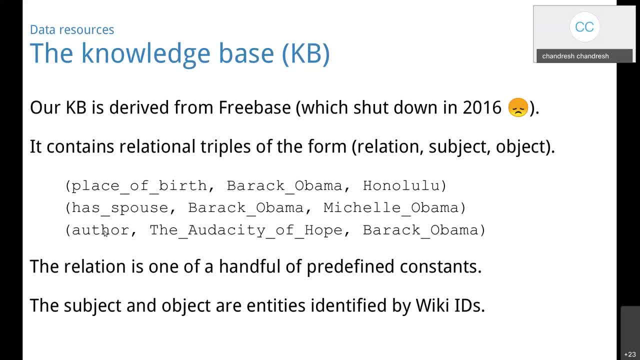 a label for our uh classifier, right? so we'll see. we can pose this problem as a multi-class classification or a multi-label classification, and these relations are actually pre-defined constants. so, total, i think 17 or 16 labels are there, right? so it's a multi-class and 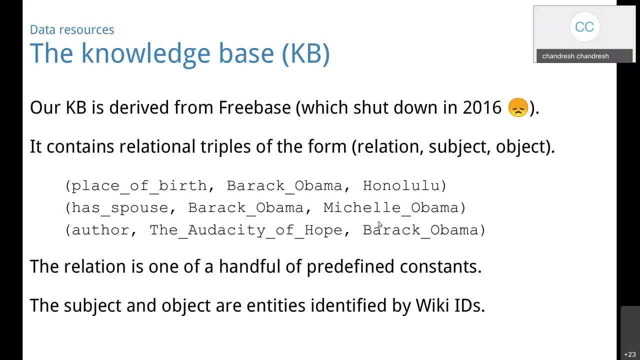 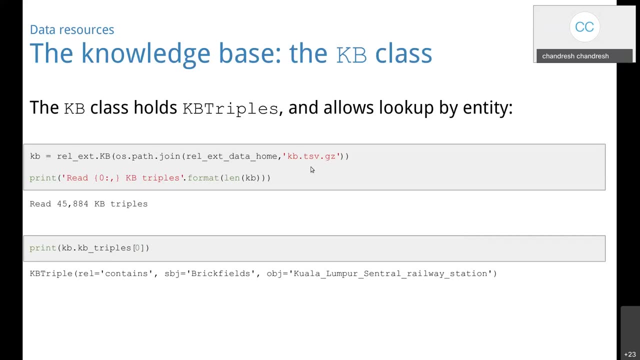 subject and objects are including entities identified by wiki ids. so these are. these are the actually wikipedia id. so if you look at barack obama wikipedia page, so last uh url would be this one, barack, underscore obama. okay, so these are the entities. so if you you. 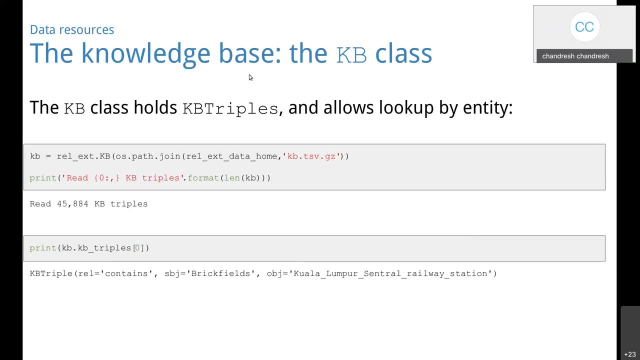 know, uh, look at this knowledge base. um right, the kb class is there, similar to our corpus class, and if you look at this triples in this knowledge base, so you'll see that there are total 45,000 triples in this kb. it's a not very big, but i think this would suffice to our work and 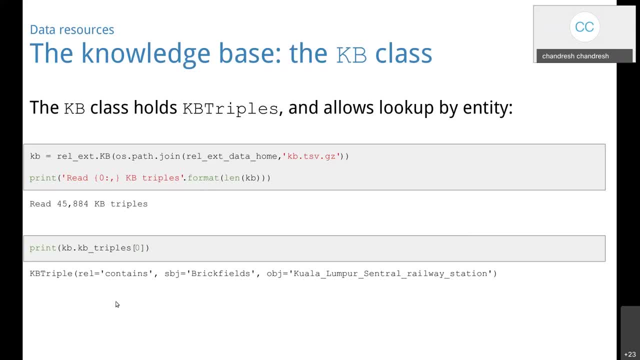 if you look at one of the triples which is there in this knowledge base, this triple is this one: uh, for example, brickfields first class is the knowledge base and then the knowledge base is the subject. object is kuala lumpur central railway station. so brickfield contains. 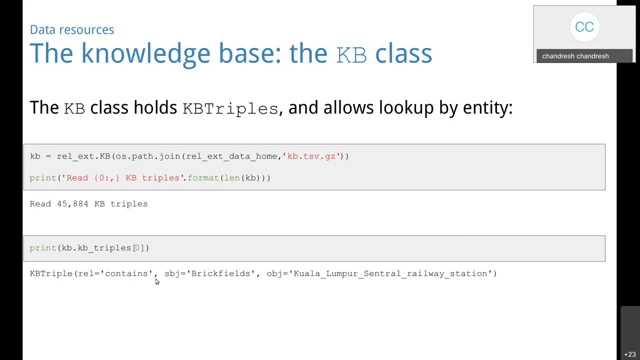 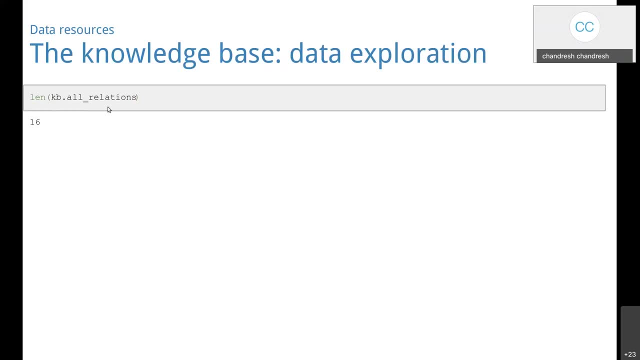 this railway station. okay, so these are the two entities, and then contains: is a relation between these two entities. all right, so if you, yeah, so total number of relation in our knowledge base is 16. that's fine, not really large classification problem. so it doesn't even know how many classes are there in image net, those who have used image net data set. 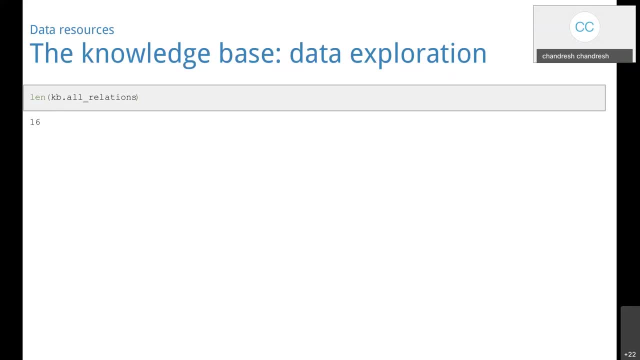 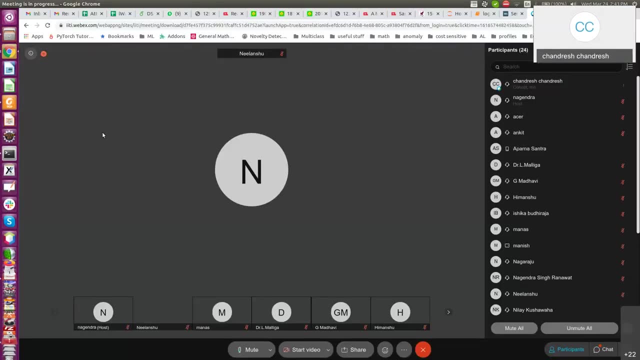 anyone here has used image net. no, okay, so in image net there are actually thousand classes, right? image net is a you know, uh, natural images of birds and vehicles and you know other stuff- bottle bag, things like that- right, so that's a image data. uh, if you look at this kb, the 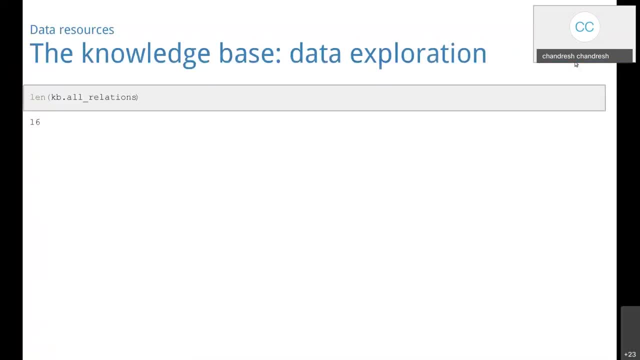 total number of relations between these two entities is 16. that's fine, not really large. number of relation is 16. okay, not very huge compared to image net. so these are the actually 16 relations which are present in our knowledge base. so what we want to do is take sentences. 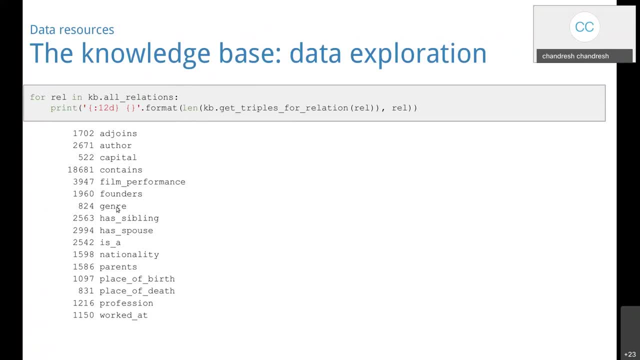 from the corpus and label them with these relations, right, so these are the frequencies of the relations uh present in the uh yeah knowledge base, i guess okay. so there are, i guess, uh, these many entities which have these relations. okay, so this frequency is telling you the entity pair which have this relation. okay, so some contents you know, frequency is very. 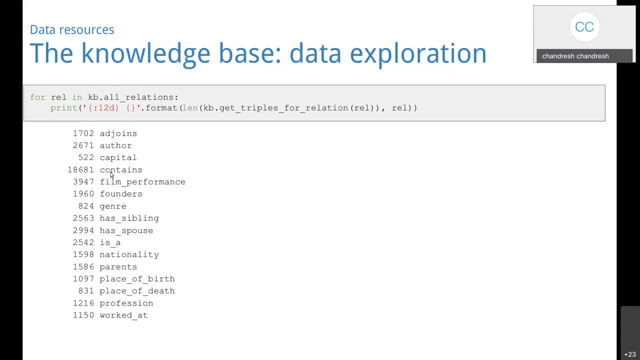 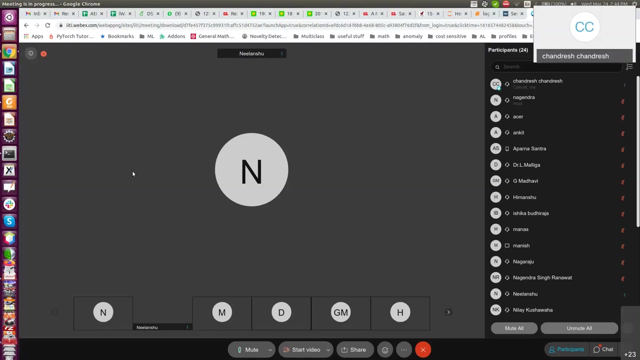 huge. so there are lots of entities which have this uh relation. yeah, okay, so far, i hope people on track. anyone lost here? no, sir, okay, clear, okay, very good. anyone else would like to say something so that i can understand? okay, people are following because the idea is to make you feel comfortable rather than bored or overwhelming nila. let me ask nila. 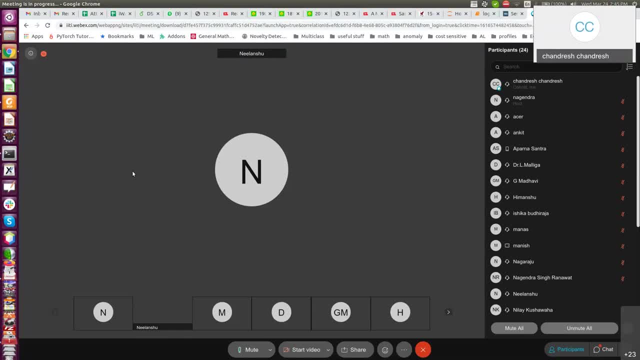 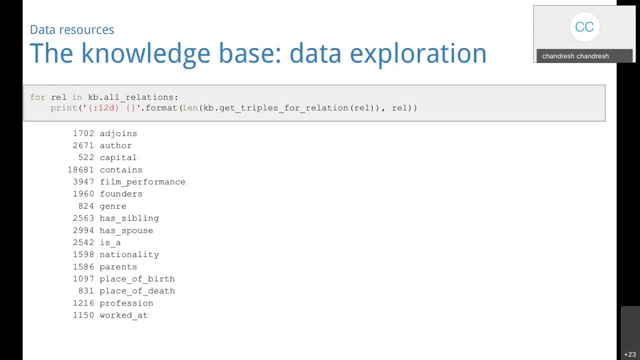 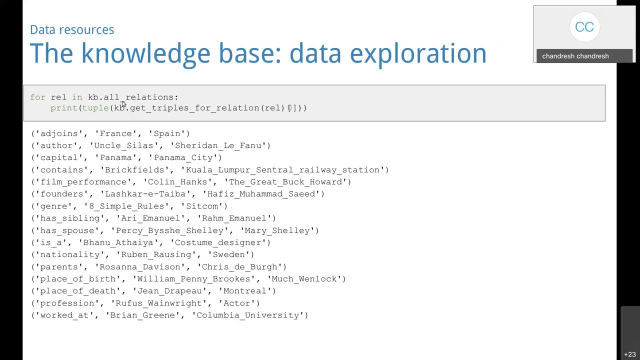 nila is not saying anything anyways. so yeah, i hope things are clearer. uh, let's, let's move on. um, so we are still looking around our knowledge base that we have, okay, so if you try to find all relations, so here we are printing. but let's say, i want to understand which two entities have this. 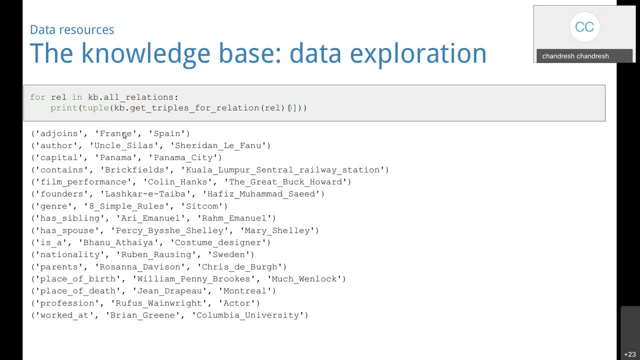 relation adjoined, right? so you see that france and spain are. they are adjoining country, so adjoined relation is there? similarly, uncle silas and sarah did leave. fanu has this relation. author, so it's. maybe it's one of the two, so it's one of the two. so it's one of the two, so it's one of the two. 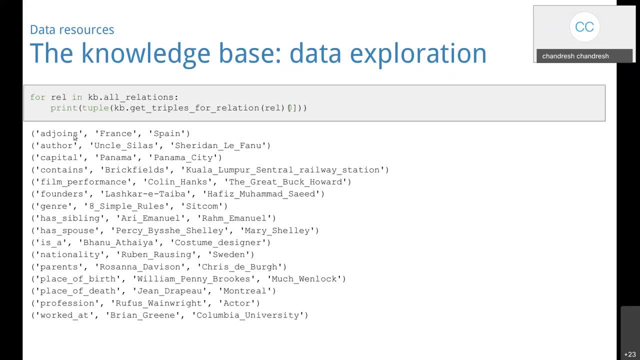 this is author is the book. so you can see, uh, some of these relations are actually bi-directional, right? so if france is adjoining spain with this relation, you can also flip this so you can say: okay, spain, uh, is adjoining the france, so same relation might hold in both the direction. but 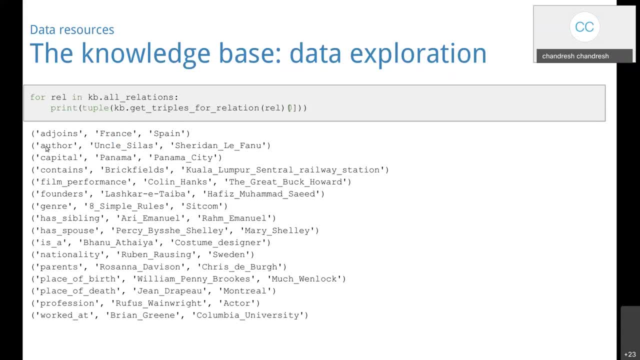 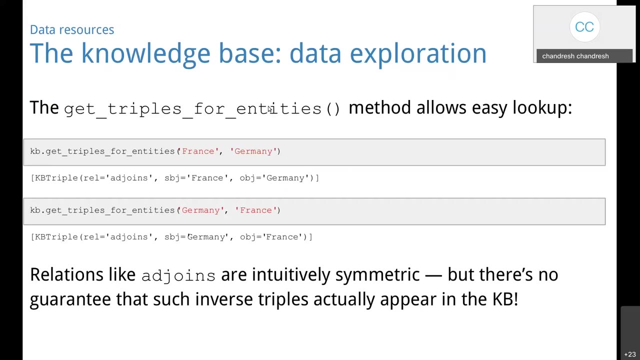 in other cases, for example, in this case, uh, this relation will hold one in one direction, right, so that's the thing. uh, okay, so, so that's the idea. um, so, further looking and digging our knowledge base, uh, we are doing data exploration. it's always good idea to you know. uh, go through your data, try to understand. 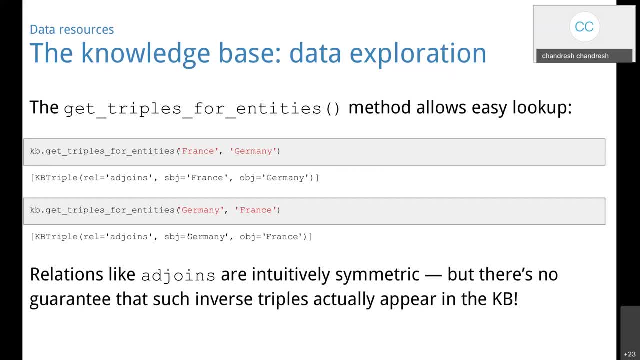 understand it as many times as possible, right? so this is what we are doing: we are exploring our knowledge base, looking at how many entities are there, how many relations are there? okay, so, if you see, um, yeah, so here, in this case, france and germany, uh, have this adjoined relation, and if you just 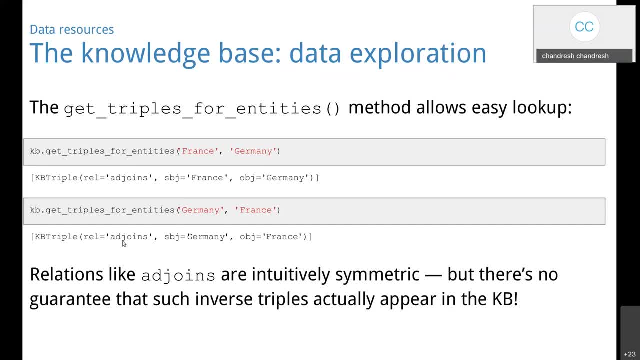 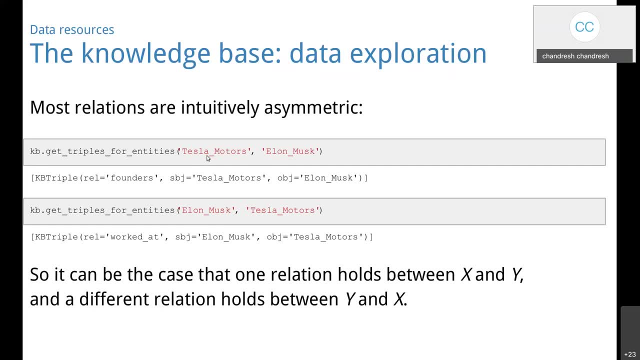 flip germany with france, then same relation holds right. so relation is symmetric. but in other case are the different relation might hold, for example, tesla, motor, ilan, mass, in this direction? the founder relation is there, but if you change uh, first entity with second one, and so on. 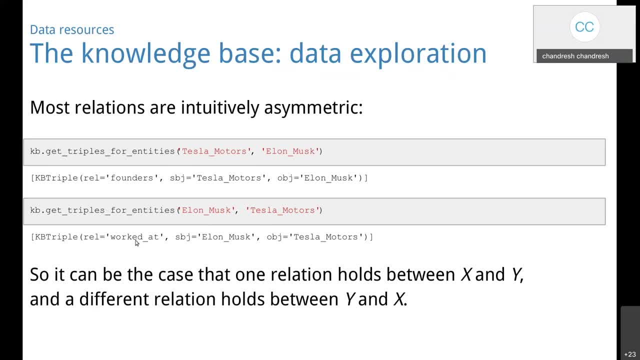 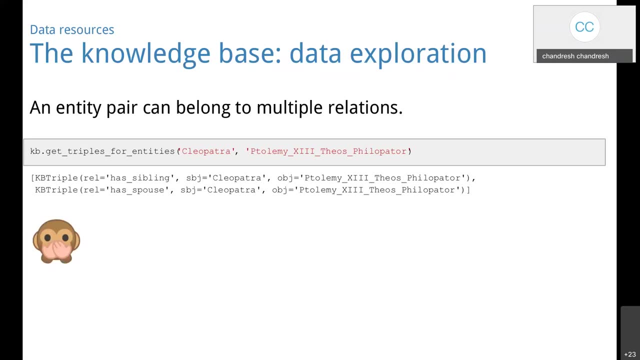 then worked at. relation is coming right, so relation is changed now. so this is very important: that you do not rely always that all relations is metric right. so if you flip, relation might change. okay, um further, an entity pair can belong to multiple relations as well, so if you 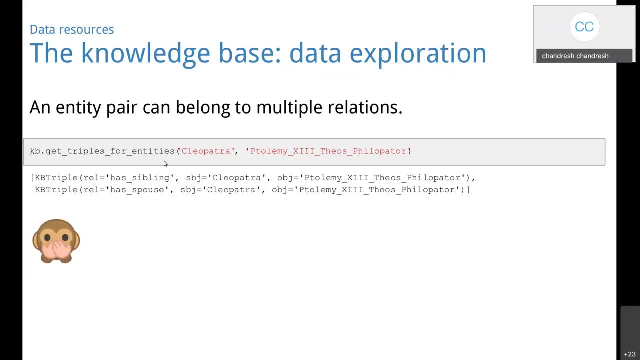 try to extract triples which have multiple entities, uh, multiple relations. so here you see that these two entities have relation, has sibling as well as has spouse. that's very strange relation. so same entity, pair, but they have different relations. okay, so it's a multi-relation triple. 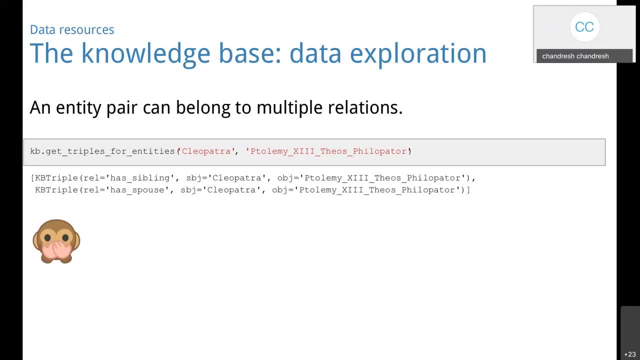 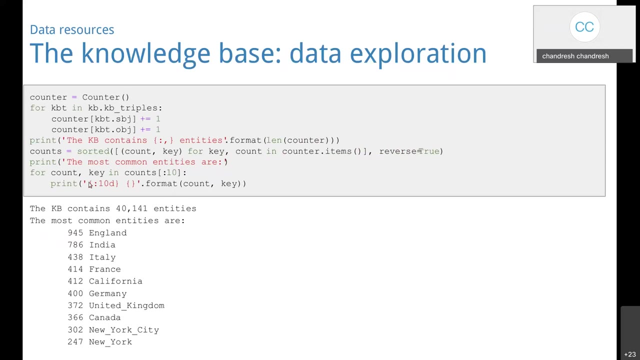 all right. so the such kind of these are called data nuances. that they are not. you know. uh, they thought the machine learning techniques to perform well, okay, um, yeah, so if you further explore your data then you will see. uh, yeah, total number of entities present in the kb is 40 000 around and the most common entities are: 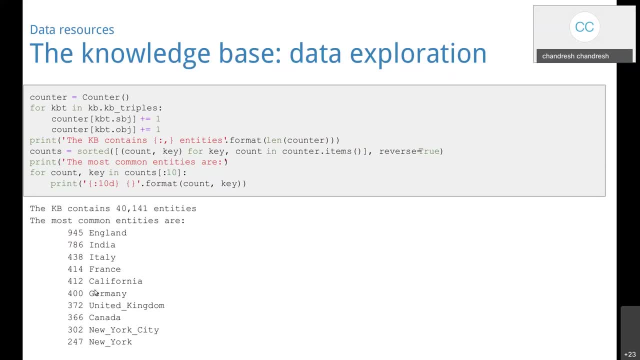 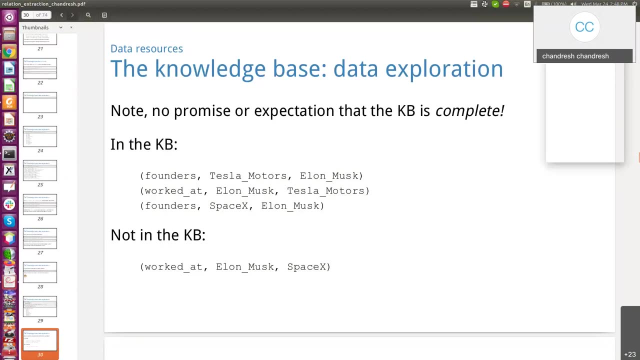 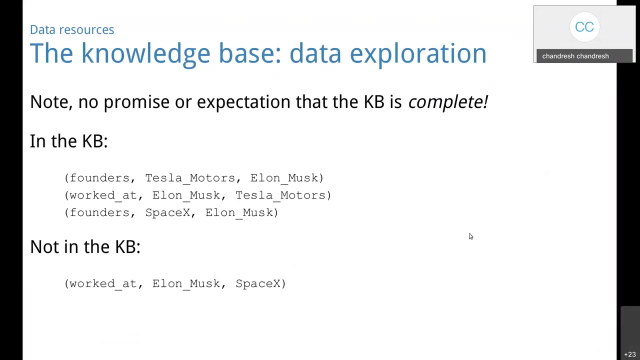 like country names. okay, so it's very simple. let us how many, how much time we have. we have still good amount of time, i guess 15, 25 minutes. good, we have time, i'll not skip very fast. so yeah, so in our knowledge base we have the. 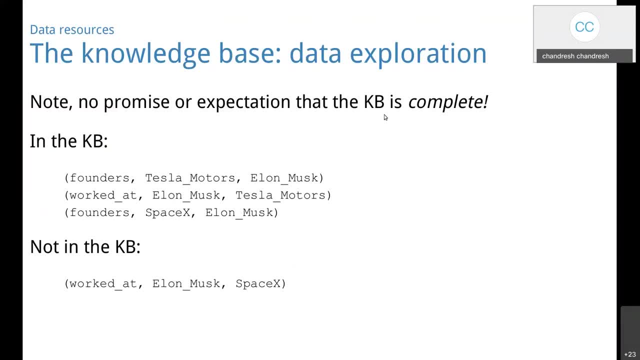 there is no promise or expectation that the kb is complete. okay, as i said, not all triples can be found in the kb. right, for example, these triples are present in the kb, but this triple is not present. so if you have a sentence with these entities, then you will miss uh this relation. 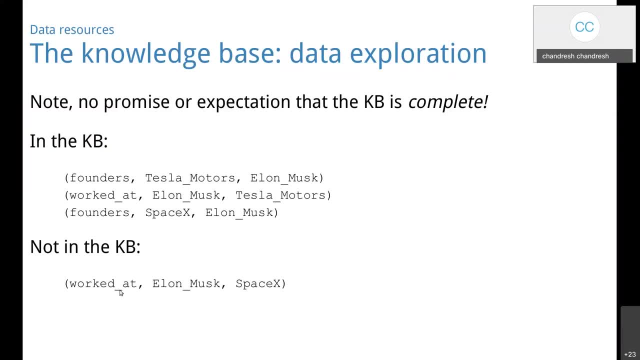 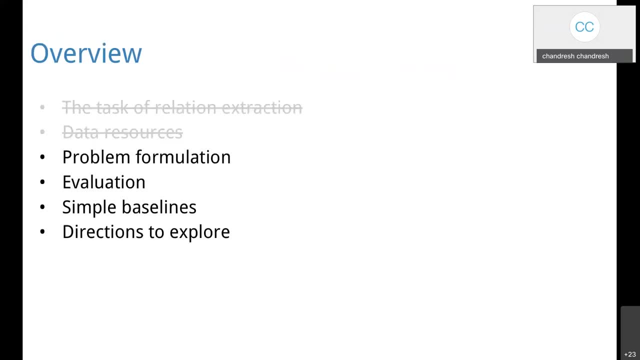 okay, because this is not present in the kb. okay, so that's the drawback, um, yeah, that you have to cope with. okay, so, having understood the problem and data resources, let us move on to understand the problem, how to solve this problem. right, so, we understood the kb, we understood the. 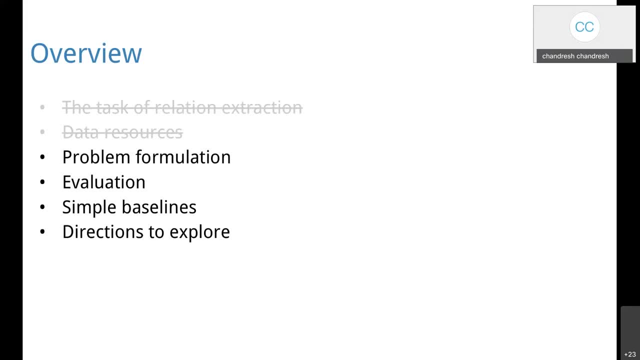 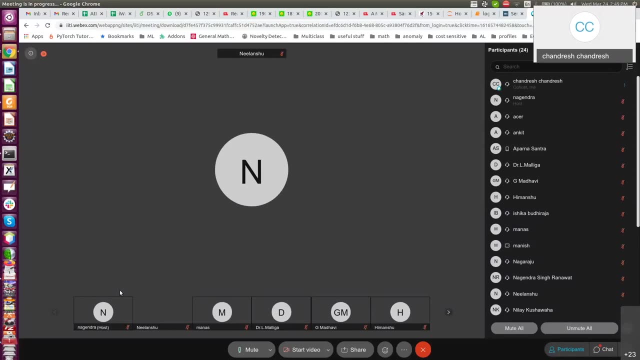 corpus. now we are going to uh solve this problem: how to actually do the relation extraction. okay, i hope people are so far still not lost, so things are okay. okay, so let me ask him: anyone would like to say something? nilansu is waiting. yeah, he's still awake. maybe others are lost. 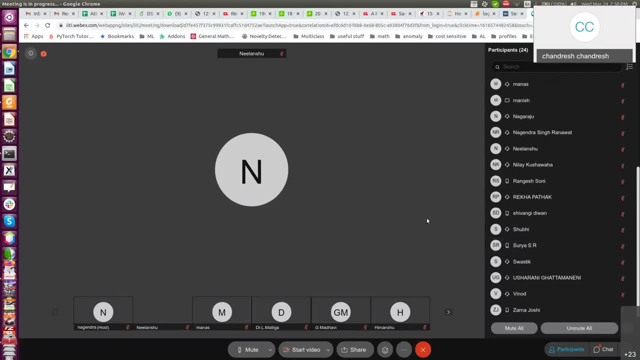 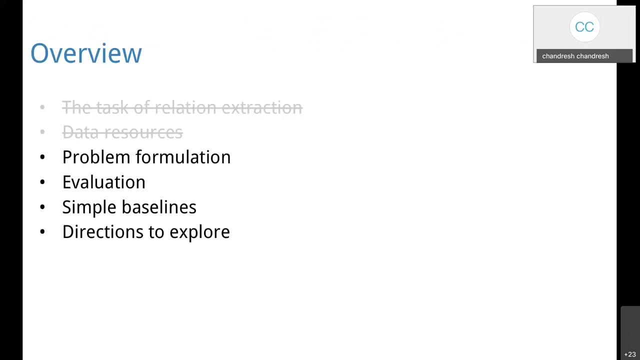 let me ask him if he's there. yes, sir, sir, i'm able to understand, okay, very good, those who are following. very good, this that keeps me motivated, if you're following, all right, so let's understand the problem formulation. um, so we are trying to understand our input and output and then we'll join the corpus with the kb. then we'll gather. 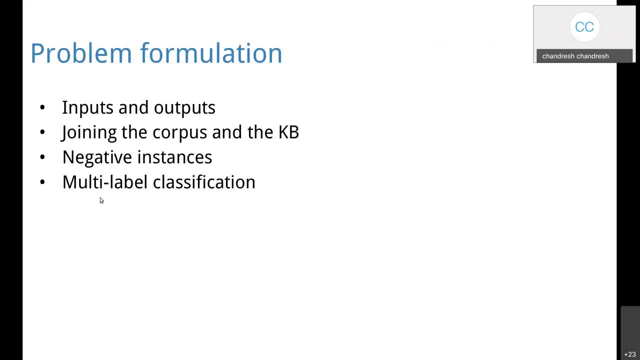 negative sentences and we'll pose this problem as a multi-label problem, as we saw earlier, right? uh, same entity pair might have multiple relations and then you'll get the negative. so each relation is a label. so if there are multiple relations, so i want to predict all the relations, right? so that's why this is a multi-label problem, okay. 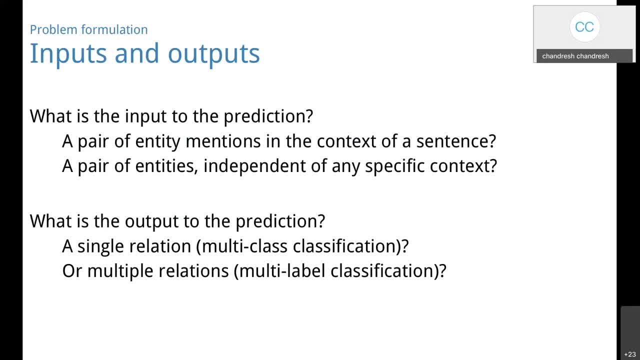 um, yeah, so what are the input and output? uh, so what is the input to the prediction? predict input: is this a pair of entity mentions in the context of a sentence, or a pair of entities independent of a specific context? okay, so there are two ways we can give. 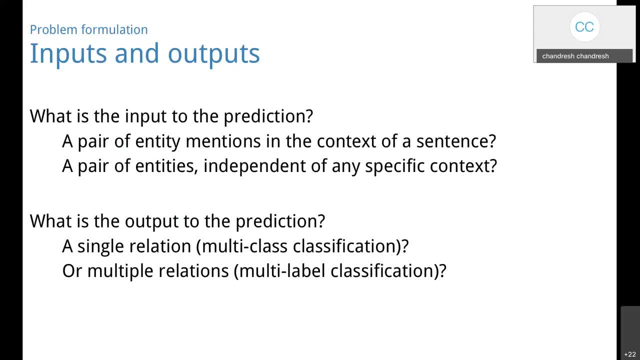 the input. either we give the entity mentions, given the context, like left of the word, right of the word, middle word of those entities right, or i can give just the entities rather than the context, okay. and similarly the output can be a single relation, i can just predict which class. 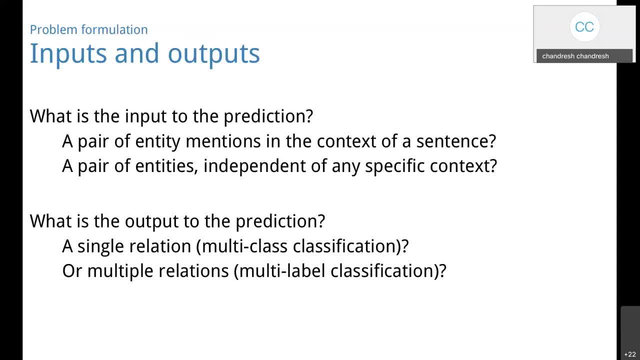 out of 16. you classes, remember each relation is a class, right? so in if i want to do multi-class classification, i will just predict the one, those relation, one of those relations, or i can predict multiple relations. so you have these choices right. you can formulate this as a multi-class or multi-label. 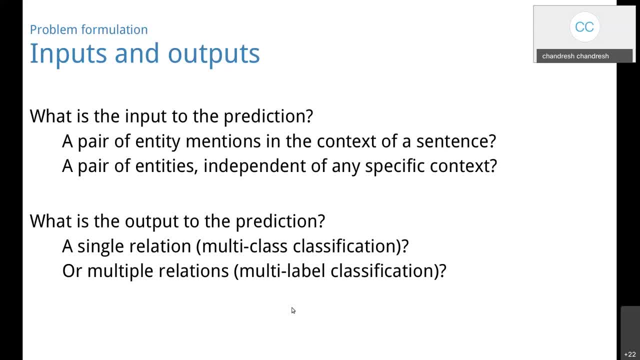 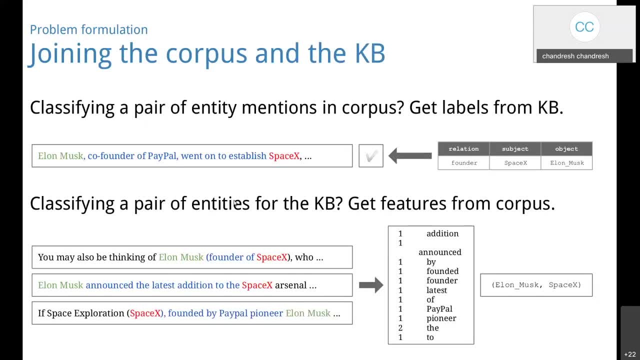 problem very simple. i hope this is clear. let us move on. so this is very important: joining the corpus and the kb. yeah, so what we want to do is that we want to classify a pair of entity mentions in the corpus. so what to do? get the labels from the kb that we have been doing right. so take this. 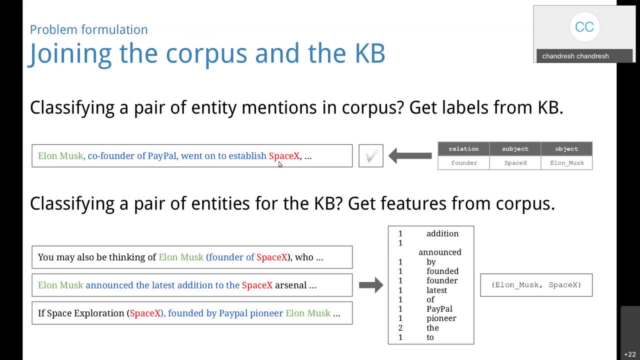 sentence, extract the entities via named entity recognition and then, uh, search for those entity in your kb. if there is a relation, then label it as plus one, okay, and and if you want to classify a pair of entities for the kb? so this is what is happening, can you see? 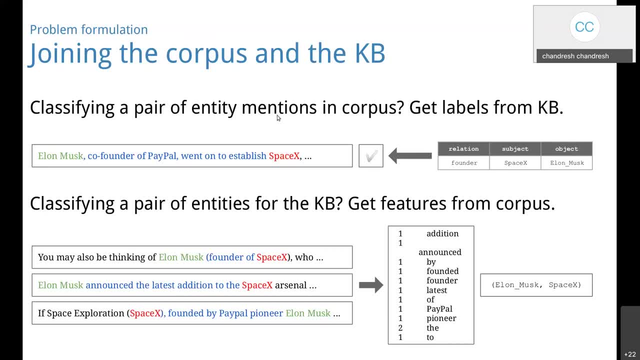 both the things are. we are doing things in both the direction. so if i want to classify a pair of entity mentions in the corpus, so read these two sentences very carefully. here it is saying corpus. so i am looking at sentence from the corpus. extract the entity. look for them in the kb. 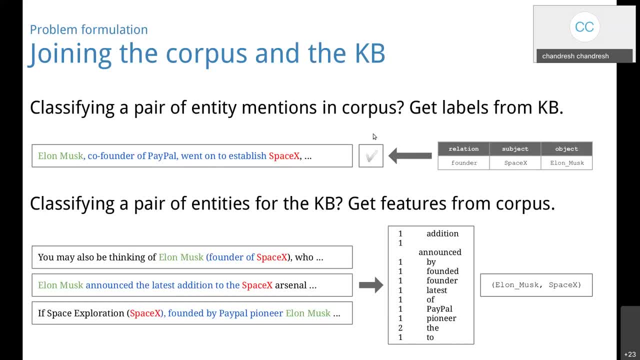 see if there is a relation. if yes, then put a tick mark. okay, so we want to help our kb as well, because kb is not complete. it doesn't contain all triples, right? so if i want to classify a pair of entities for the kb, let's say, if i have these two entities, i 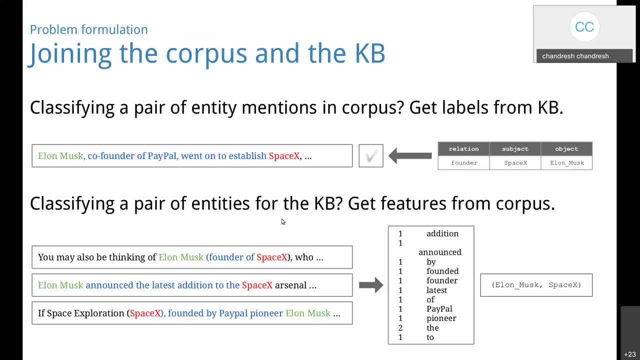 want to know the relation, what to do, right. so i want to classify these two entity pair for this kb. so get features from the corpus. so remember these other other words: left, middle and right. they can be used as a feature for this. this entity pair, right, so you can use the sentence in the corpus to build. 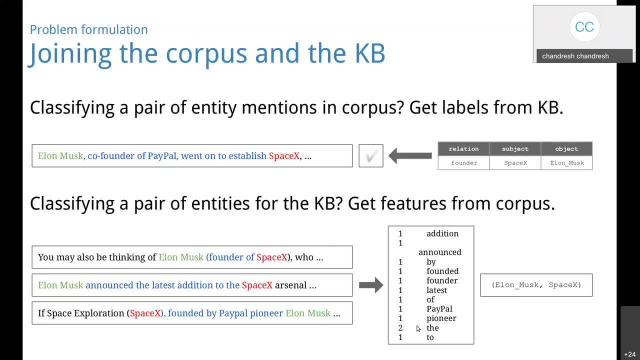 a feature. right, i guess these are the frequencies of this word: addition appearing one. the is appearing two. okay, so these are the frequency. you these take these three sentences and build a feature vector. so here, feature vector is just a frequency. you take individual word and count the frequency. 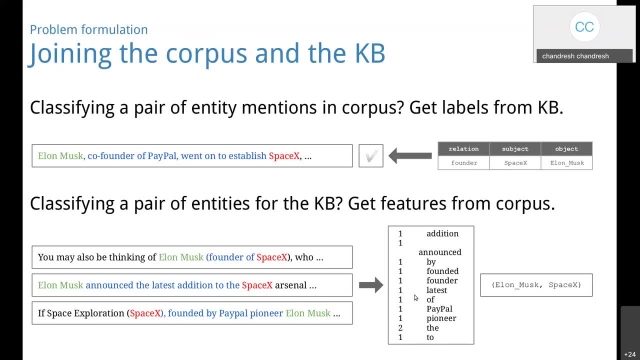 that's it right. so that's how? uh, kb and corpus, they are helping each other. okay, so this is an intelligent way to connect these corpus and kb, right? uh, i hope this slide was not very confusing. let me know if it was before i move on. people say yes, no. 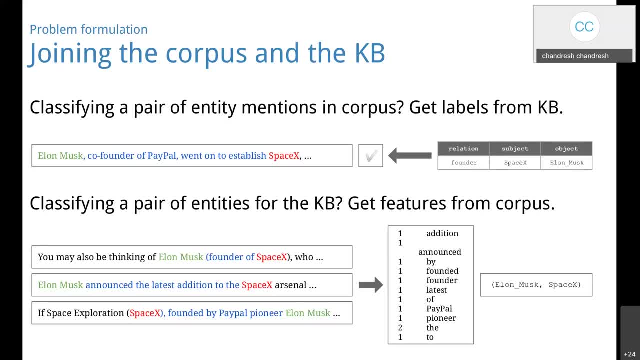 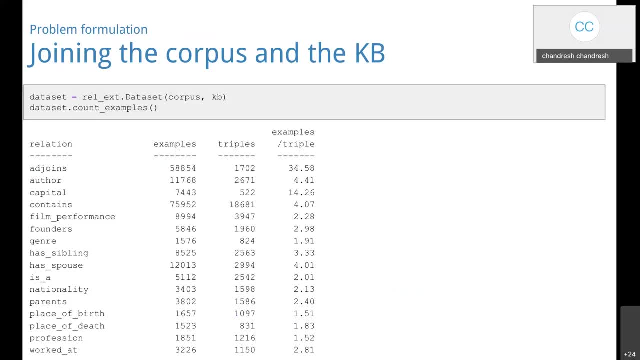 okay, looks like people are lost now. okay, don't worry, you can always go through the slide or the video. okay, so here, uh, we are going to join the corpus and the kb. so if you do that, um, so what happens is this? uh, you look at the relation adjoint: the number of examples in the corpus. 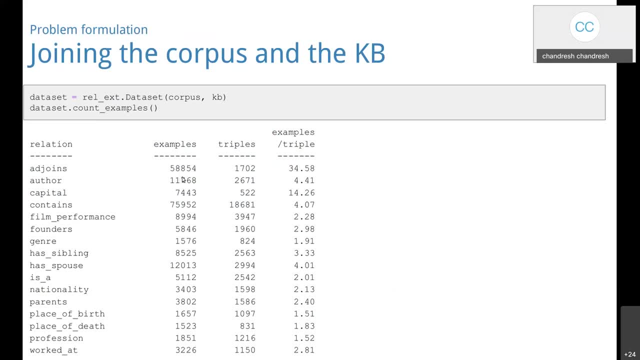 which contain this relation is around 58 000 and the number of triples which are there with this relation is around 1700. so you can say that uh total number of examples which contain uh a triple is around 34, for example this deletion. so there are around 34 sentences. 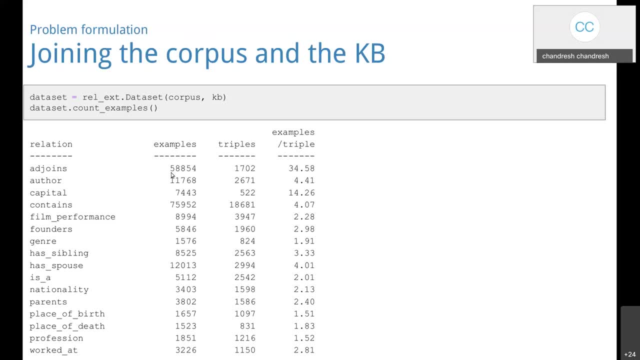 which contain uh one entity paired uh with this relation. okay, so 34 uh examples. yeah, per triple. so one triple will appear in 34 examples, right with this relation. so this is what it is saying. so can you see that number of examples per triple? it is varying a lot. for example, there are: 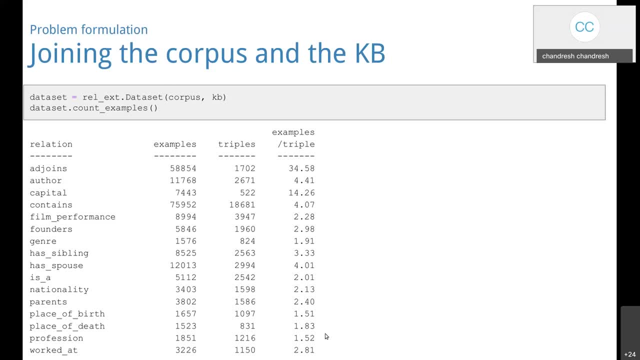 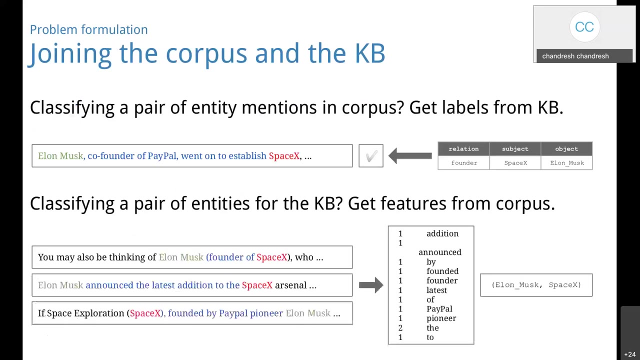 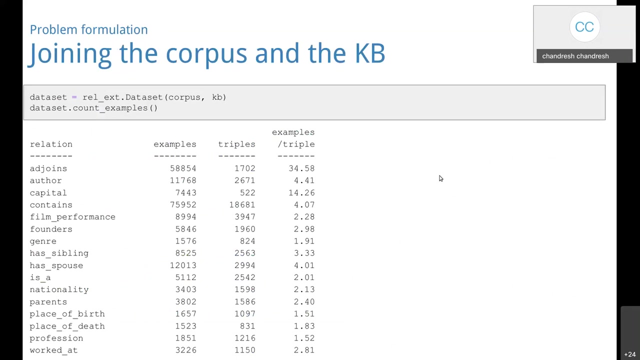 relations which appear like. number of examples containing this triple is very less okay. so that's the. you know, some relations appear more often than others. right, okay, so you are able to get positive sentences in this way. what to do with negative sentences? anyone has any idea how to get negative sentences, so here we got positive sentence, right. 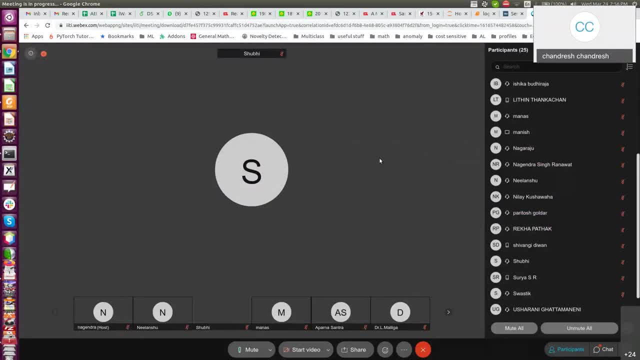 what to do with negative sentence, how to collect it, let me ask, because i want to build a classifier, right, so i need a negative sentence as well. usha rani, do you want to say something? i think she has been a regular attender. attendee- uh, not sure if she's hearing swastik. 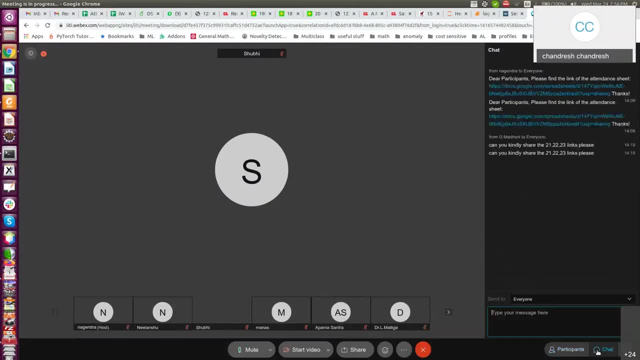 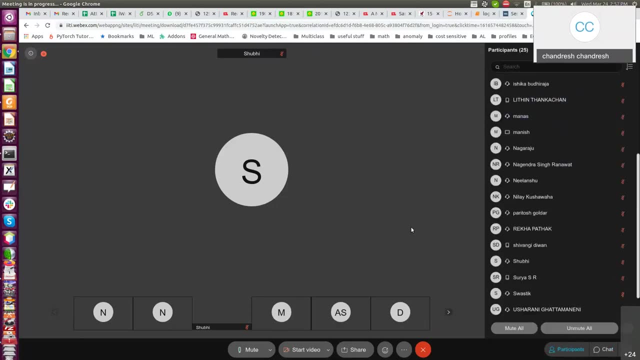 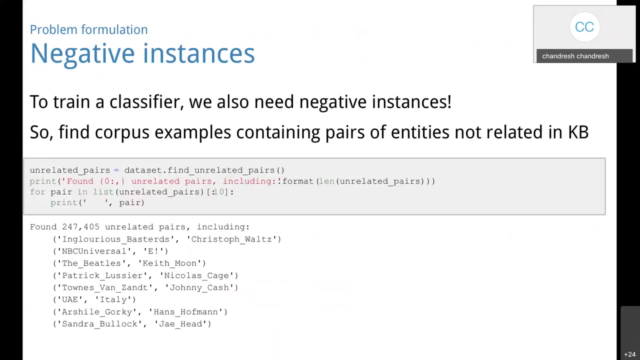 anyone wants to throw some random ideas? okay, no one? okay, no problem, let's see. um. so to train a classifier, we need negative sentences. okay, so find corpus example containing pair of entities not related in kb. okay, so we are going to look for sentences in the corpus, uh, extract the entities and see if there is a relation. okay, not related in kb. so if you search, 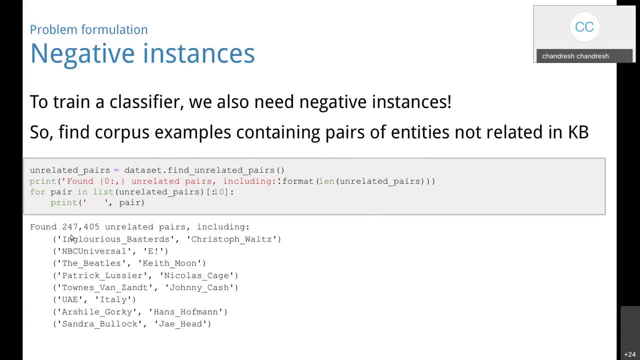 for such pair of entities. then you see that there are actually use number of entity pairs which are unrelated. Okay, so there are around 247,000 entity pairs which are not related. Okay, So you have found positive sentences. you have found negative sentences. 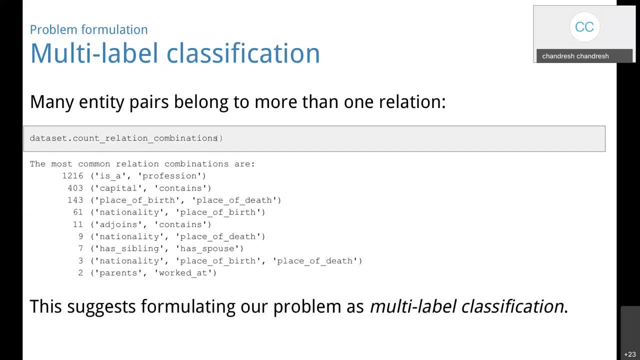 now you're good, you can go ahead and train the classifier. So. but again, since we want to do a multi label classification, so there are actually many entities which have more than one relation. So if you count such relations, so you will see that the entity Phar might be related with either. 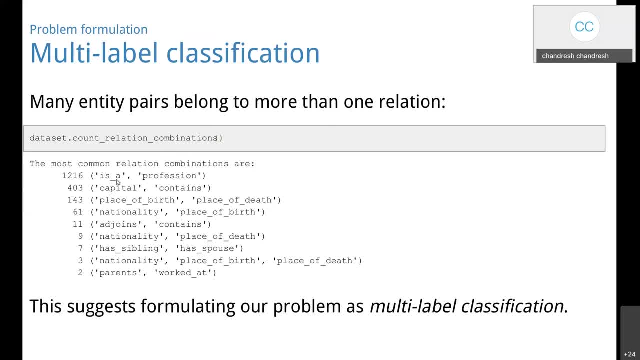 relation of progression. for example, Einstein is a physicist, Okay. Or Einstein in professionally, the physics, physicist may be right. So same relation might hold between same two entities appear, So this is the frequency of those relations, Right? So that's why we want to. 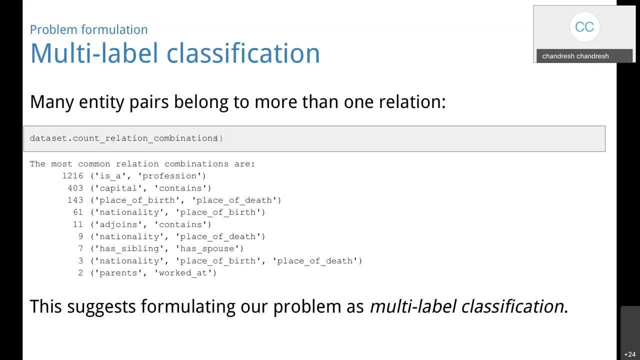 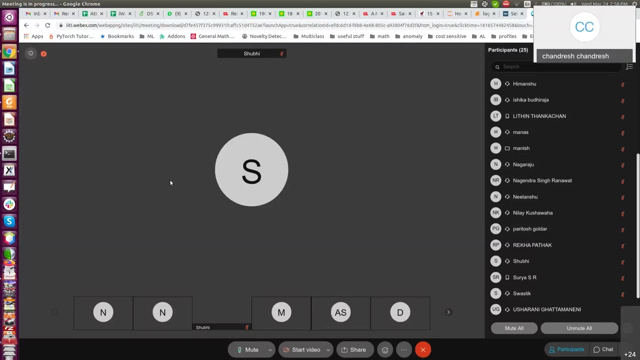 pose this problem as a vari 종, The other две multi-label classification. okay, um, so we are so far, so good. i hope nilanshu. maybe nilanshu was hearing nilanshu. let me get one voice. uh-huh, nilanshu is not there. 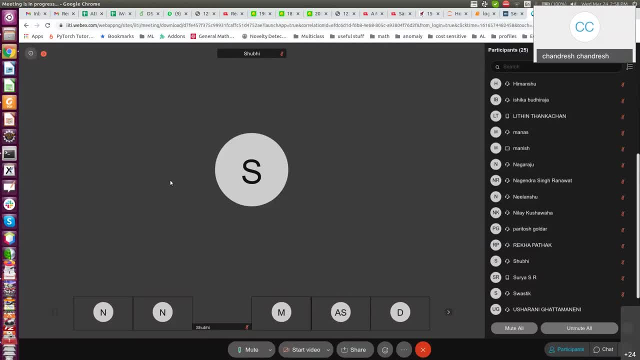 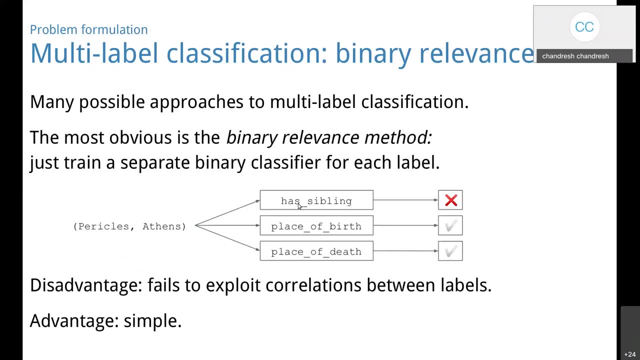 okay, so we have these relations, so we have to do a multi-label classification. let's see so there are many ways to do a multi-label classification. one of the approach is a binary relevance method in which we do a pairwise classification. so i want to predict n labels. let's say, for example, these two entities have these three labels. 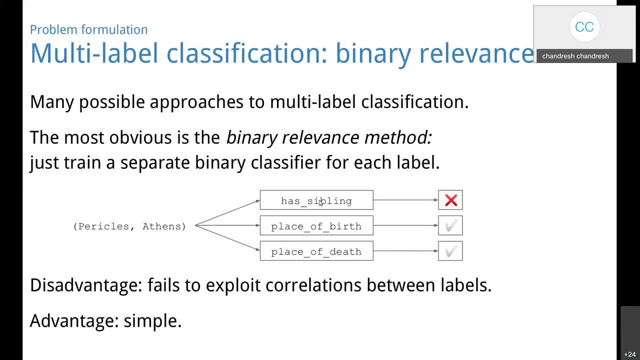 right, so we have a pairwise classification and we have a pairwise classification, so i will train one classifier for each label. so for this label, i will train one classifier. for this label, i will train another classifier. for this label, i will train another classifier. okay, so this is known as a binary relevance approach for doing multi-label classification. 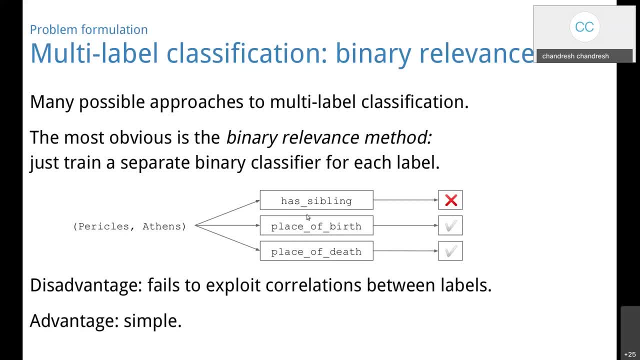 okay, you train individual classifier for each label. however, there is an issue that it fails to exploit correlation between labels. so sometimes these labels are correlated and then they become correlated, but you train independent classifier for each label, then it's not going to work. okay, the advantage is that it's a simple okay. everybody likes simple approach. 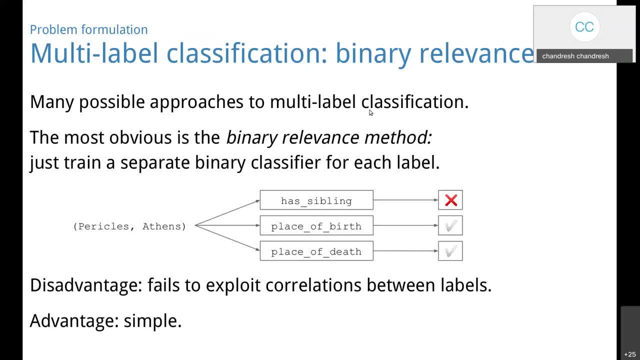 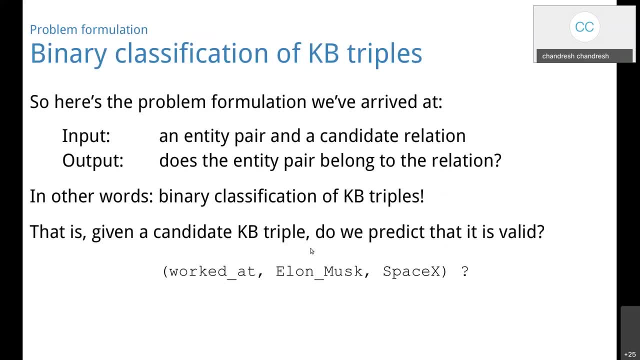 you can do that, but you might not achieve as good accuracy in case if you exploit the relation correlation between the labels. all right though. so binary classification ofκtreebuue. so input is an entity pair and the candidate relation, here and then this one. and this one have two variables, which mean we are trying to Dip. 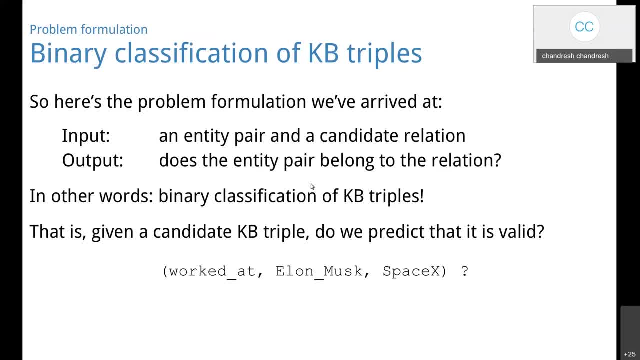 O at k transform whether the relation holds between the entity pair or not, so it becomes a binary classification problem. so given these three things are triples- uh, two entities and one relation- i want to ask my classifier: can you predict if there is a relation or not? okay, so i'm not actually outputting. 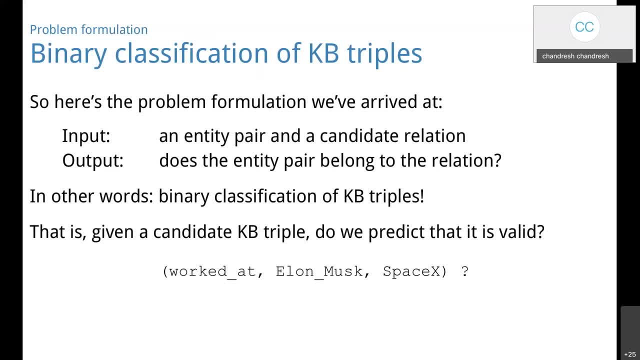 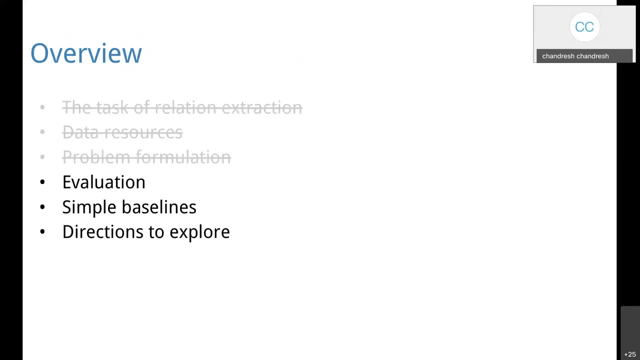 uh, you know, uh, actual relation, but i'm just asking whether there is a relation between the two entities or not. okay, so it's, this problem is slightly different, all right? um, yeah, so let us go to the evaluation. um, so evolution has this stage driven development, split the data. 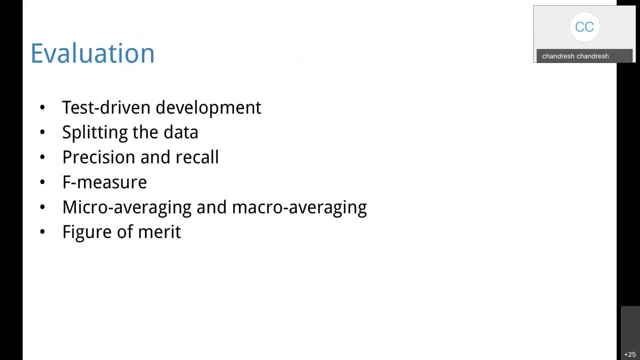 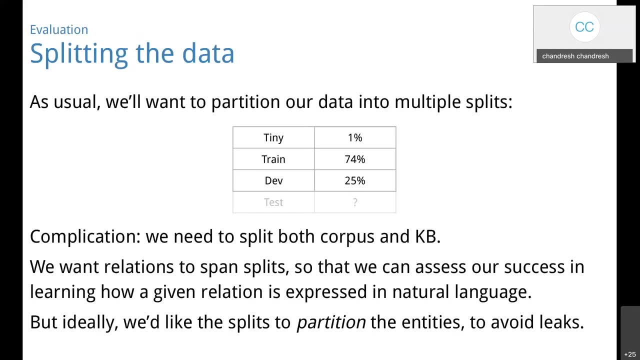 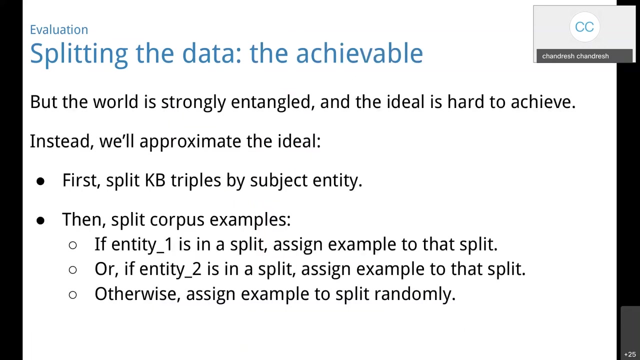 calculate the precision and recall, do f major macro averaging. macro averaging and many other steps are there, right? so let us uh skip this part. how to split the data, i think you already know, you know, train development test, um. so this is how you split the data: old kb, new kb. let us skip this one, um. so, in this corpus, the code that i will share with you, 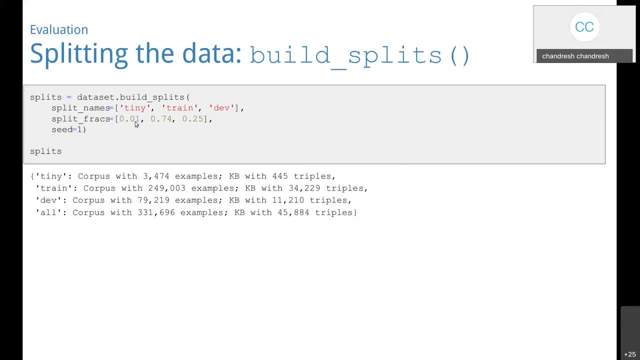 it has um routines to split the data for you. so in this case they had four split: a tiny train development and all so tiny is used to train a small model just to test whether your code is working right. so before you actually optimize your code, first you need to build the code right. so tiny data says used to. 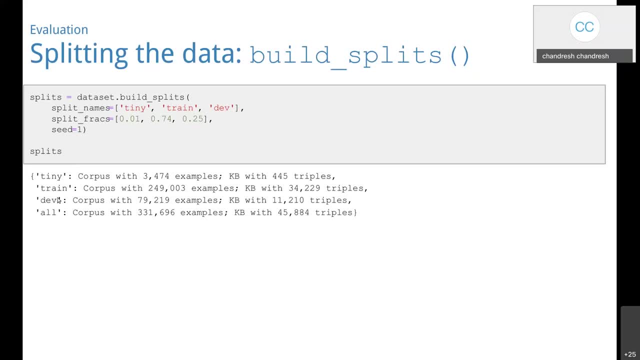 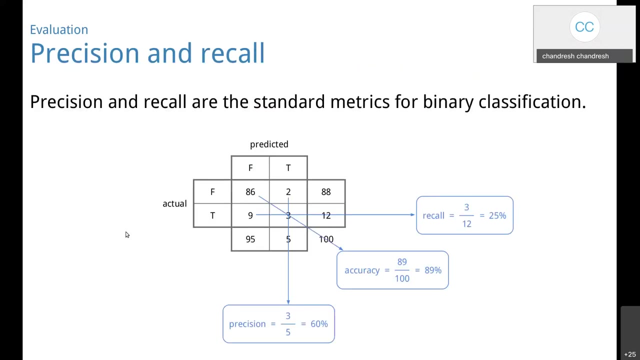 build the code. that's it. training is done on this train set, parameters are tuned on development set and actual evaluation is done on, i guess, uh, here this, uh, yeah, maybe you can go ahead and evaluate on all the data sets, okay, so so i hope people are familiar with precision and recall matrices. 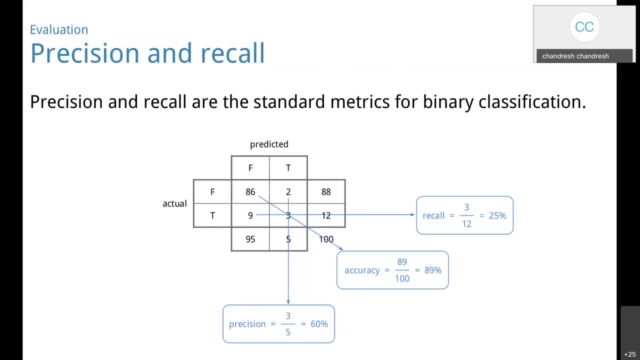 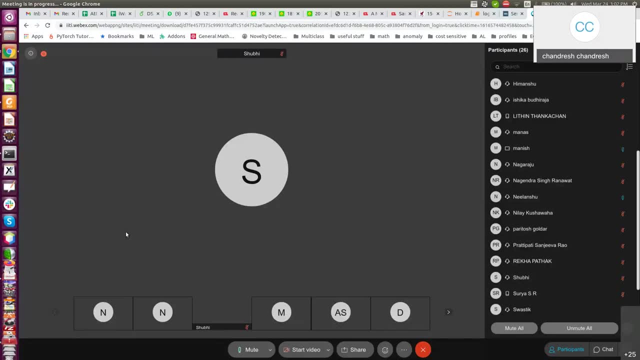 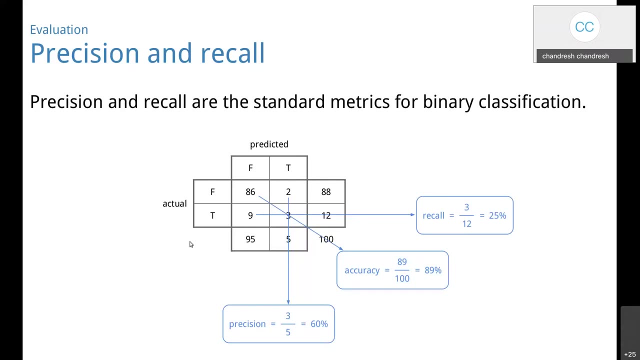 uh, anyone here not familiar with this one? what is the precision? what is the recall? yes, sir, i'm not familiar. oh, okay, let me uh explain that then. okay, so let us say: uh, i want to, um, uh, so this is the actual label. this is true and false or positive, and true is positive if is negative. 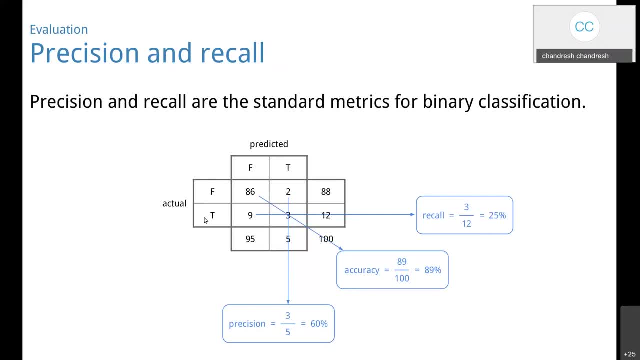 these are the predictions. prediction can be true or false, right, you can think of, this is your uh head. uh, this is the tail. this is your head. this is tail. okay, and a coin flip. so, and i want to build a classifier to predict what is going to come if i toss a point, right? so if you look, 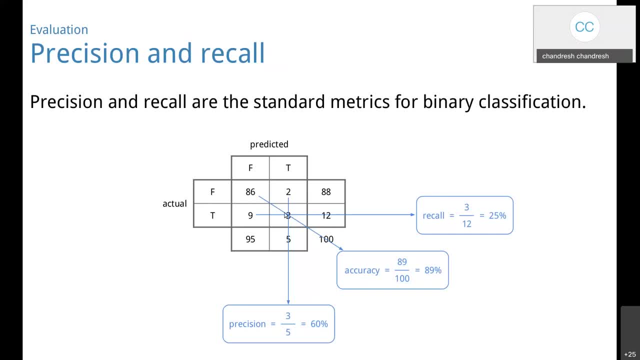 at this row: okay, t and t. this sales tell you that actual level was t and i also predicted t. okay, so this is this: three is saying that actual, uh, so total. so let me see i'll tell you what these numbers are first. so 12 is there are total, 12 heads or 12 positive classes. 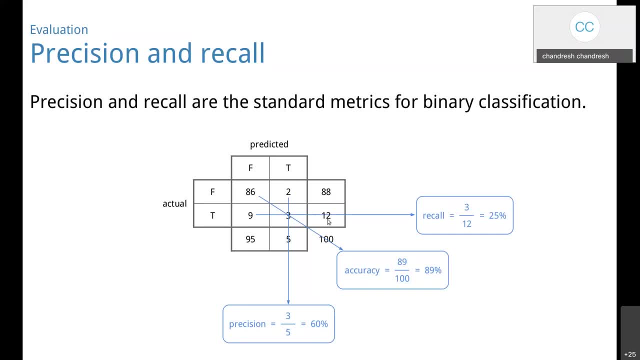 and 88 negative classes are there. okay, so these are the actual and these are the predictions. so while predicting, i am saying there are five positive and 95 negatives. okay, so if i fill my metrics, if you look at this inner matrix, okay, so these numbers are tading out of 12. 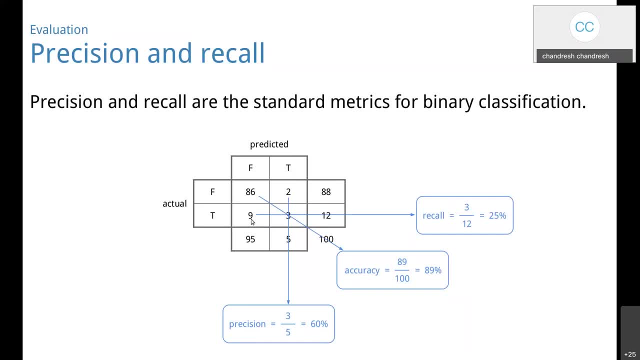 3 are actually predicted positive and 9 are negative. so if i sum, i will get 12 right. similarly, out of total 88 negative, 12 are predicted. so out of 88, uh, negatives, 2 are predicted as positive and 86 are predicted as negatives. okay, yes, these numbers are clear, i can. 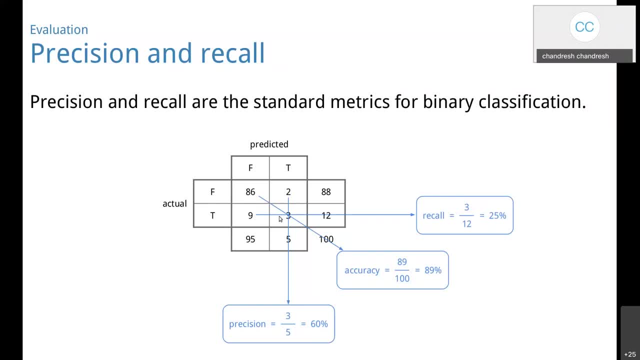 what these are. yes, yes, yeah, so, yeah. so if i want to calculate the accuracy, so accuracy is nothing, but you sum the actual prediction, correct predictions. so what are the credit predictions? so i, true class or positive class is predicted as positive. so so you take the diagonal entry. 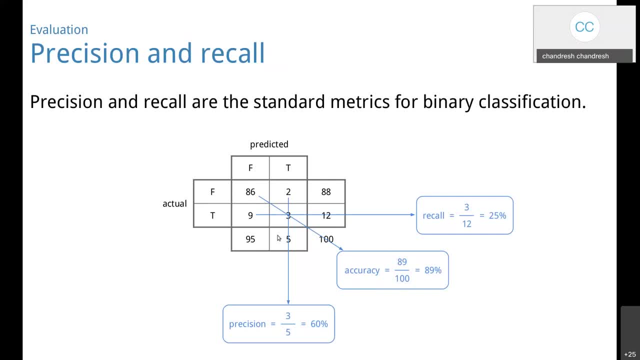 and sum them: 86 plus 389 divided by 100. so total, there are 100. examples, right? if you sum all these entities, it, all these numbers, it will be 100. or you, if you just sum these, there will be 100. this rows is 100 and so on, right? so no matter how you sum the total number, 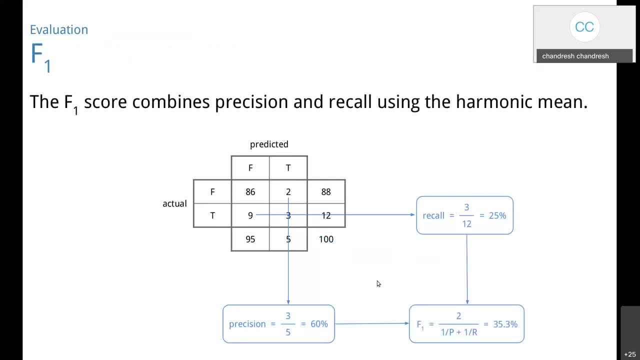 of positive negative is 100. so you actually calculate the accuracy. you divide your correct predictions divided by total: uh, examples: right, yes, accuracy is this number and recall is nothing but 357. your positive predictions: uh, fraction of correctly predicted positives. so fraction of correctly predicted. so total positives are total 12. okay, and out of 12, how many are actually correctly? 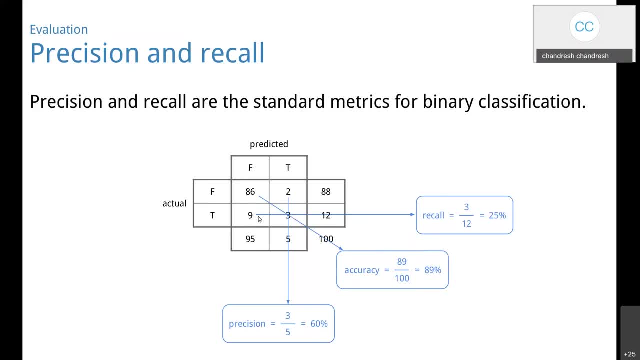 predicted 3, only right. remember, this is a false prediction, right, so actual label was t, but i predicted f, okay or negative. so this is an incorrect prediction. this is incorrect prediction. this is correct prediction and this is correct, okay. so recall is nothing but, uh, fraction of. 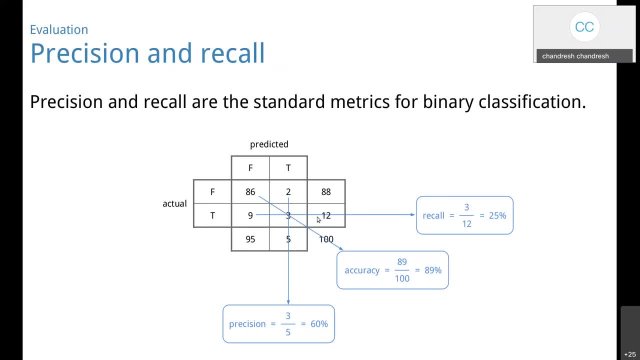 correctly predicted positive. positive is total. and what is the fraction of that which are correctly predicted? only 3. so recall is 3 over 12, okay, and precision is this one: okay. precision is just numerator of precision and recall is the same 3, 3, but here the denominator changes, so here: 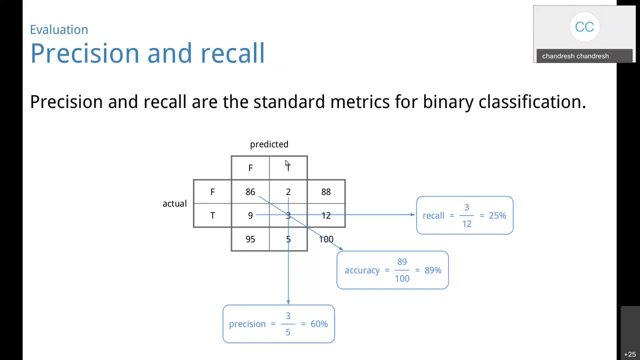 denominator is nothing, but you look at the predicted positive and count how many are actually correctly predicted. so fraction of uh correctly correct predictions, correctly predicted positives, okay. so total positive predictions are 5. so 5 is total positive prediction, right? so in this column, if you look right, t is my uh true column or positive class, right. 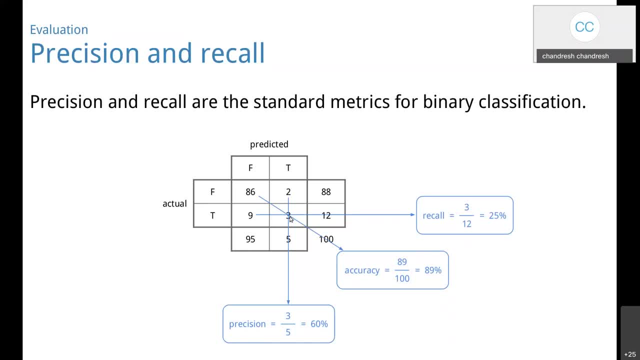 total are five. and what? out of five correct predictions are three only, right, remember this. two is coming from because, uh, negative label was predicted as positive, so this is incorrect, right so total, uh, positive predictions are five. but out of five, only three are actually correct, right so? 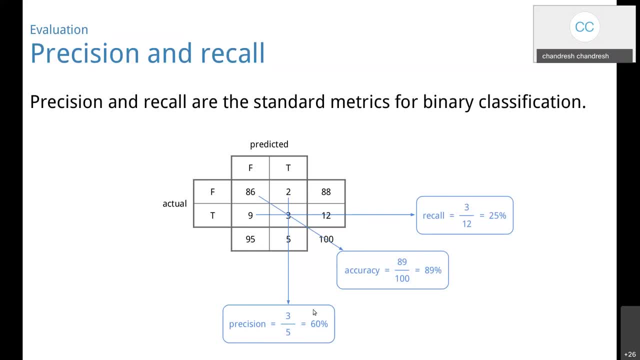 three by five is a precision, so precision is more towards the predictions. so what is the fraction of uh correct predictions? okay, uh, positive. fraction of uh positive predictions. i hope, uh, this was not very too much verbose. yes, people, i hope you are able to understand precision and recall now. yes, yes, okay, so, and f major f1 score is nothing, but you take the harmonic mean. 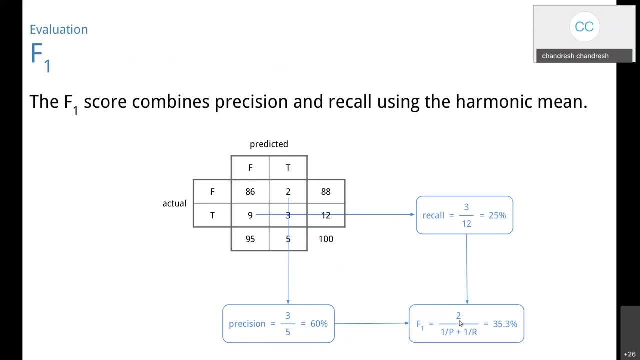 of these two, recall and precision, harmonic means two divided by one over p plus one over r, where p is the precision or can recall. okay, so that's your f1. so f1 actually takes into account, uh, both classes, positive or negative, so it's a better metric. while reporting the classifier performance, we report precision, recall and f1 as 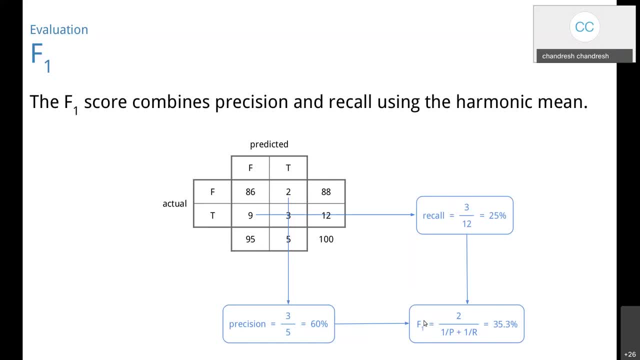 well, rather than just precision or just recall. but again, it depends on the application. so, uh, while i am was an IBM So application I was working on, they were more interested in high precision. So it depends on the application which metric you want to report, right? Sometimes I'm interested. 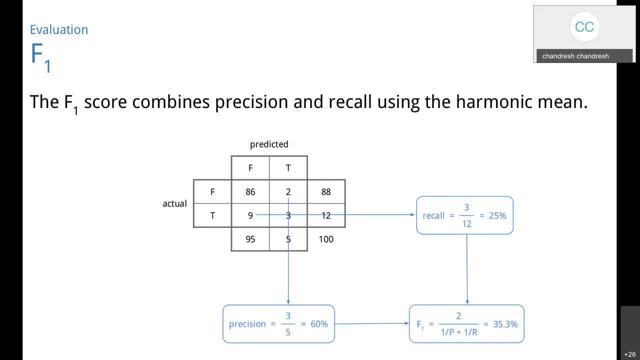 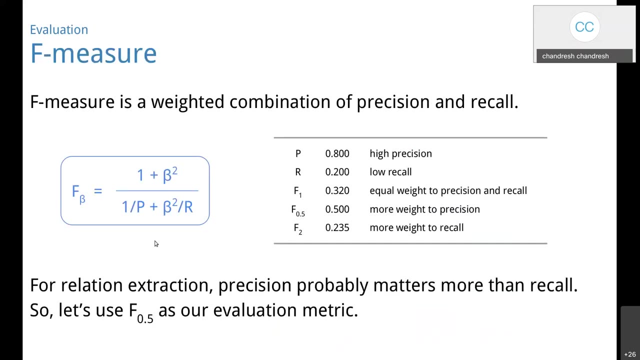 in just recall. sometimes I'm just interested in precision And in medical domain I want, I want to have both high precision and high recall. Okay, So it depends on the application. So so there is a. more F1 is one score, So more generalized F measure is known as F beta. 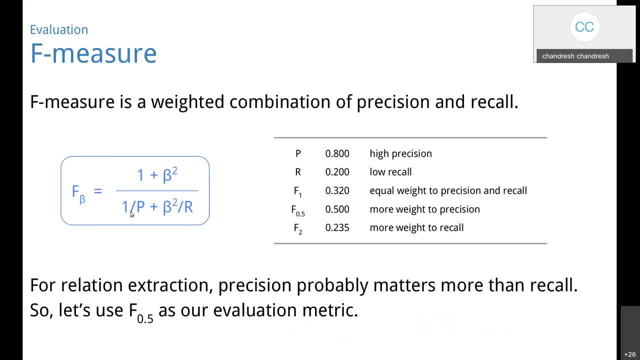 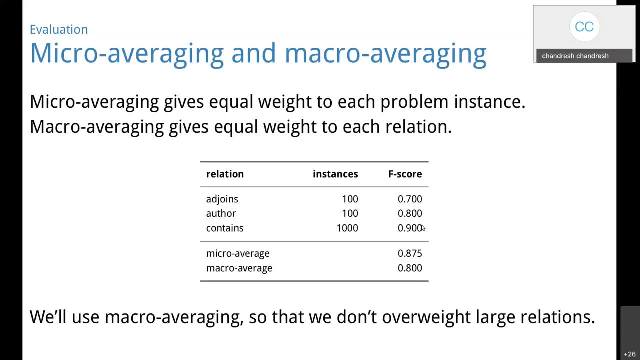 So F beta, you can set beta equal to one or point five or any other number you like, any real number, right? So you can look at this slide, let's not go into this one. So yeah, so if you run the multi level classifier using, let's say, binary classification technique, 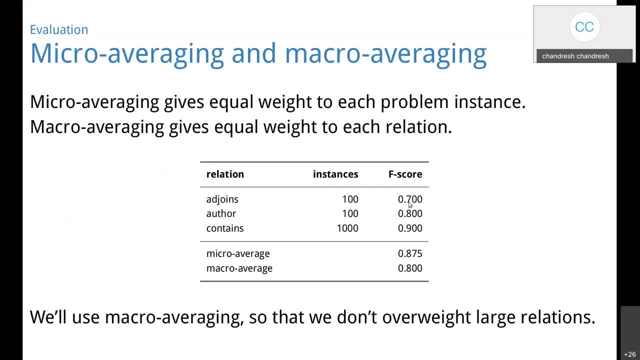 So you see that adjoint relation has a F1, F2, F3, F4, F5, F6, F7, F8, F9, F10, F11, F12, F12, F13. So we have a score of point seven. author relation has point eight. contains: has point: 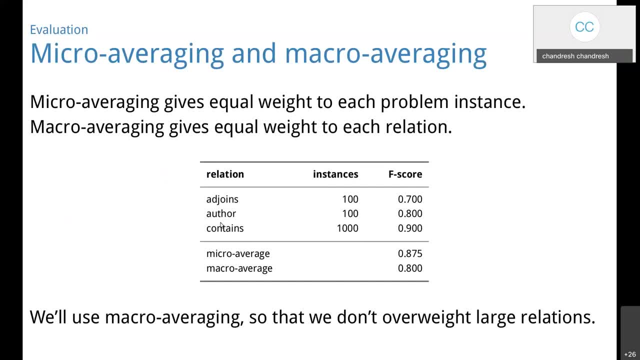 nine. That's a really good actually. So this relation is very correctly predicted. it has really high score. So more number of instances means higher one. can you see, if you have more repulse, more sentences, then you are getting better F1. So that's the idea. Micro. 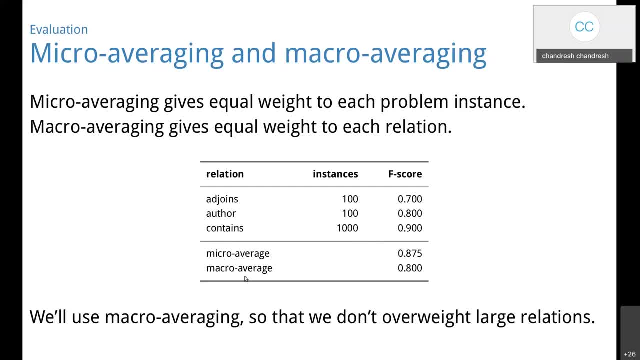 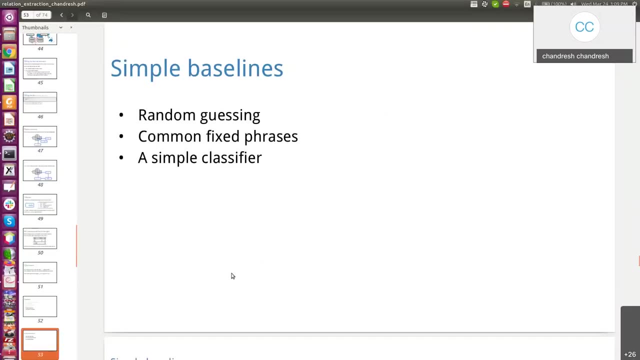 and macro average or other matrices used, especially when you have class imbalanced data right? i suggest you look at any article which explain in detail what are micro and macro average of precision, f recall or f score right? so yeah, let me see what is the time. i think we are close to. 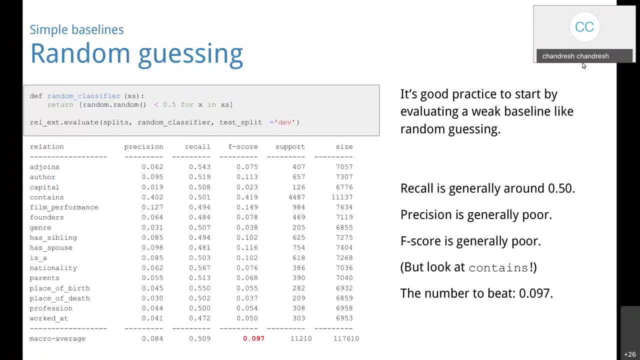 the time. let me see if i have something else to show. yeah, so this, this is the table. uh, if you do the binary classification of your data set, then random guessing, random guessing. if i randomly predict the relation, then your f score is really poor. it's just 9.7 percent. really bad, right if? 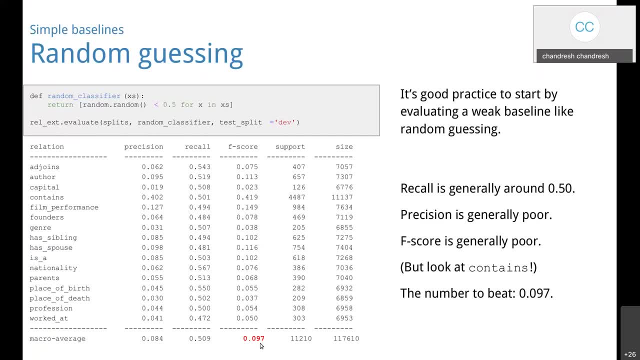 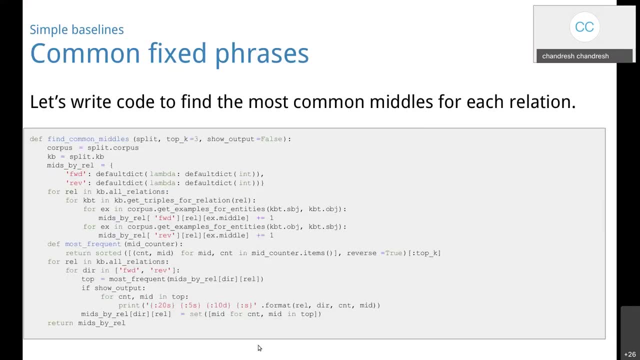 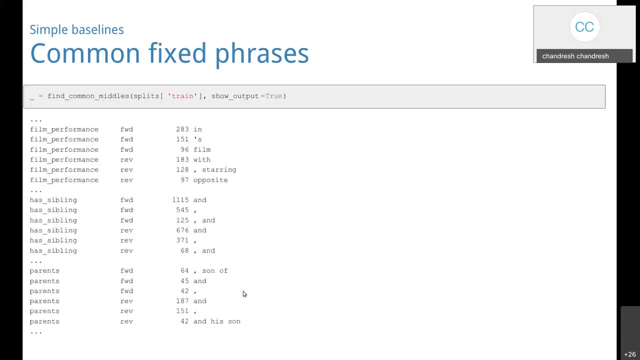 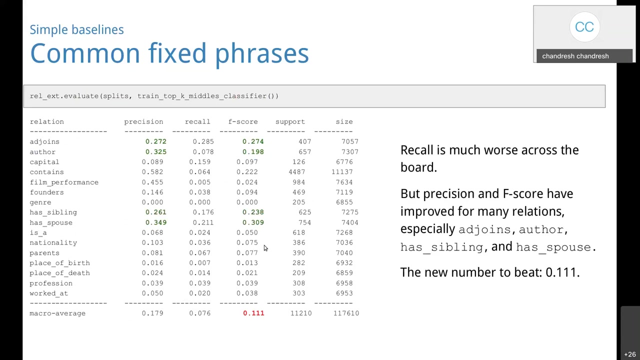 somebody asks. i mean, if you ask a person to randomly predict the label relation, it's a 9.7. really bad, okay. if you just uh write some code, okay, like this: okay, um then some common fixed phrases, uh, then there are some fix as well, which has been done here and you took lack of time not gonna explain, but with some fix, uh it. 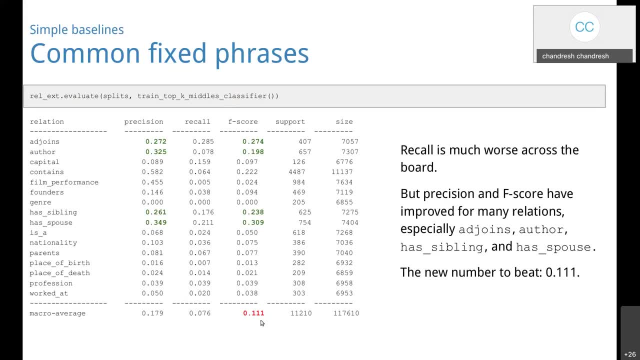 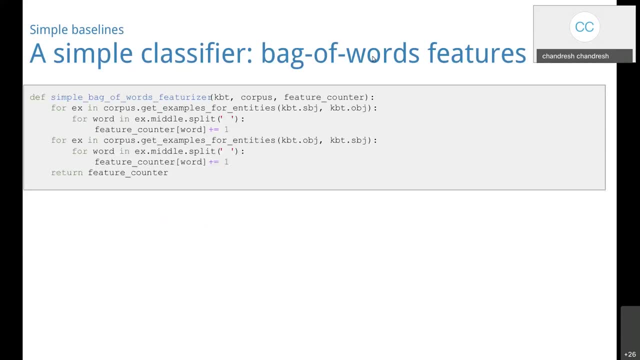 has been lifted to 11.1 percent, which is better than random guessing. uh, so if you use this bag of word feature, bag of word means i'm just counting the word and their frequency. okay, so if i use this as a feature, with that feature you train the classifier, you are good, your f1.